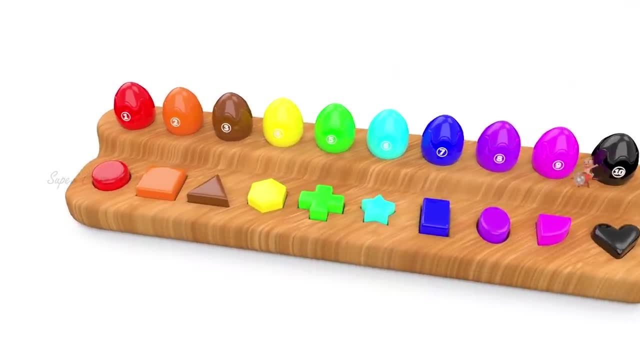 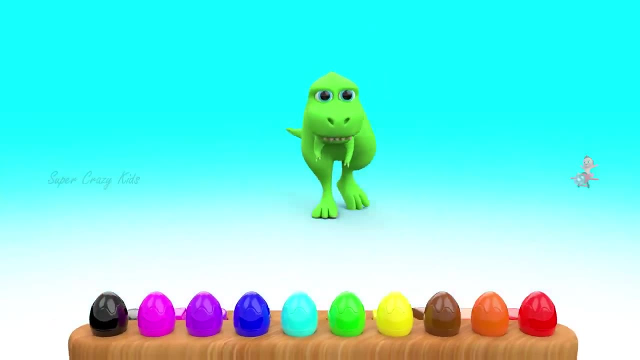 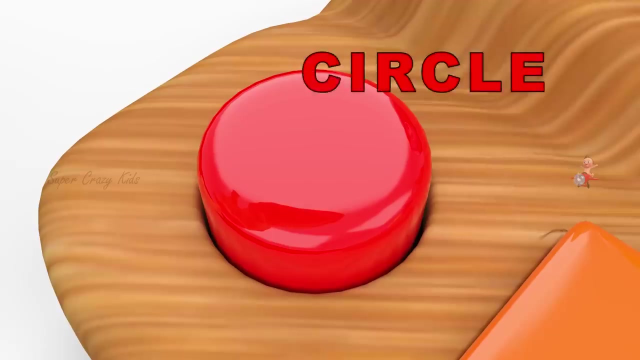 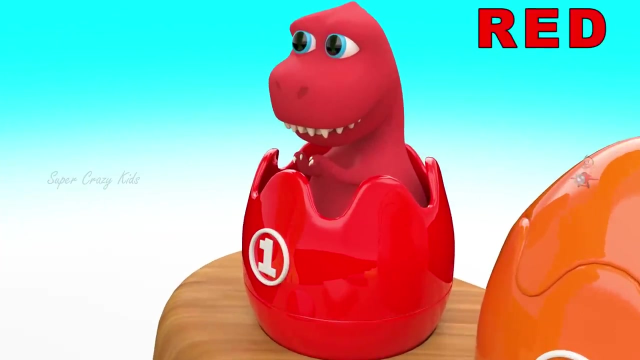 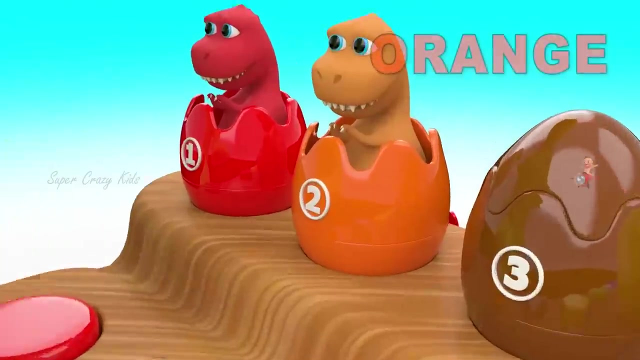 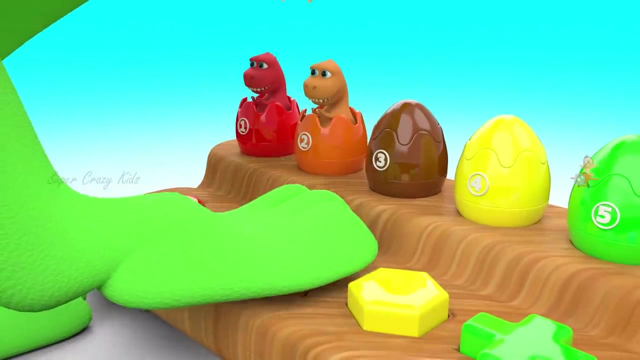 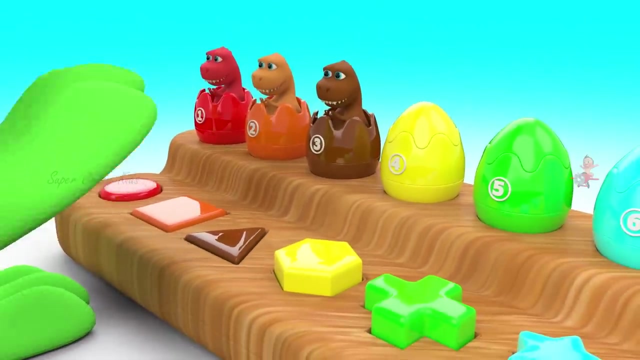 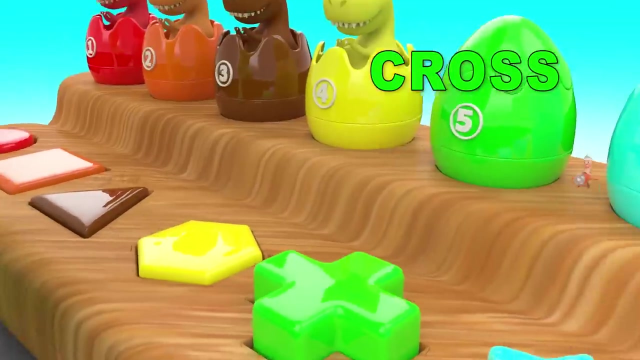 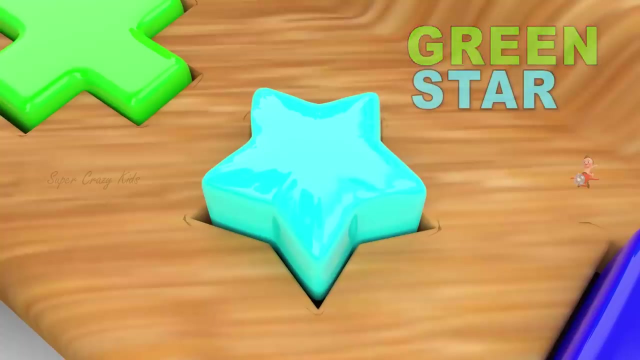 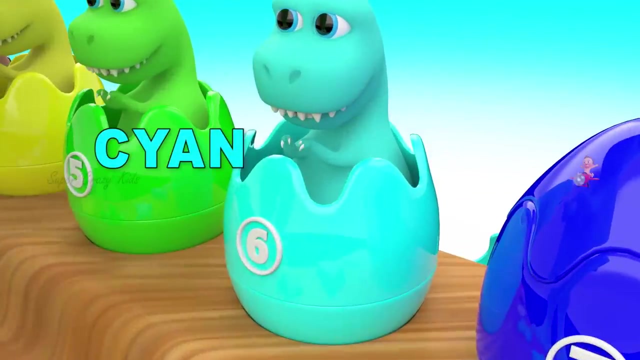 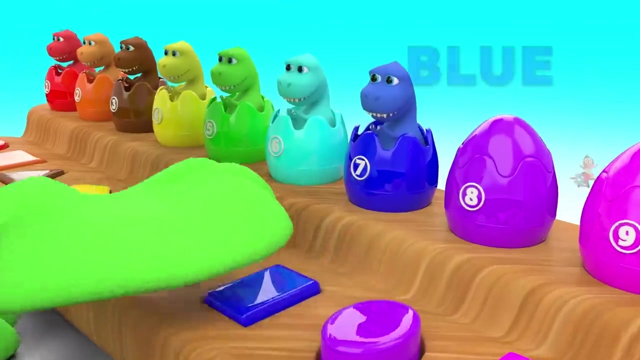 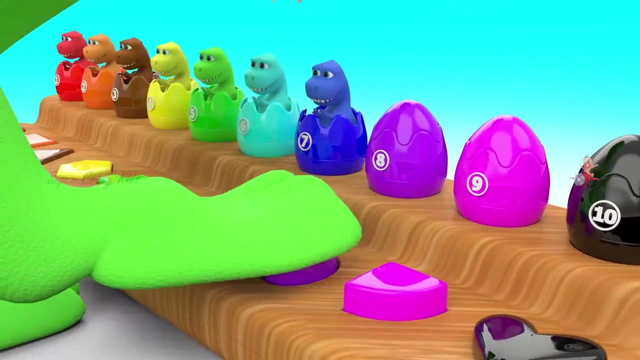 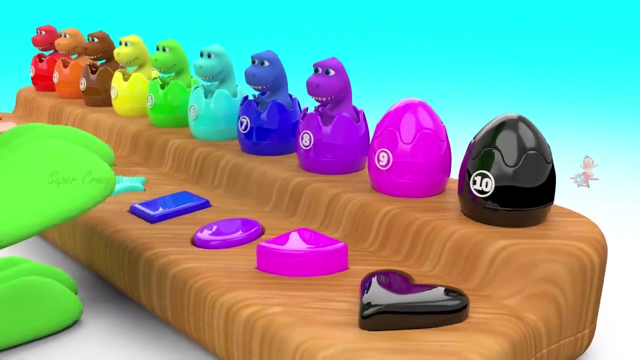 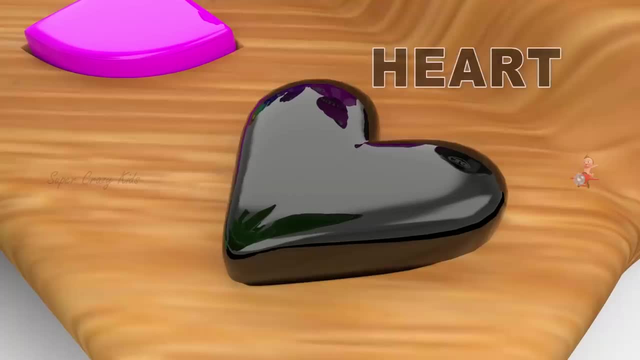 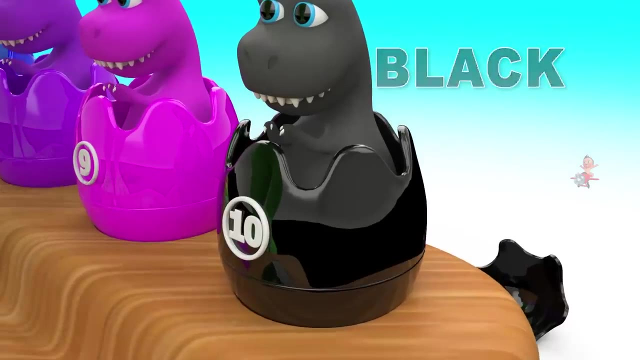 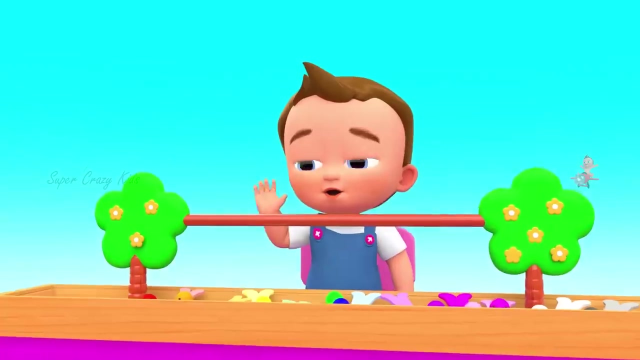 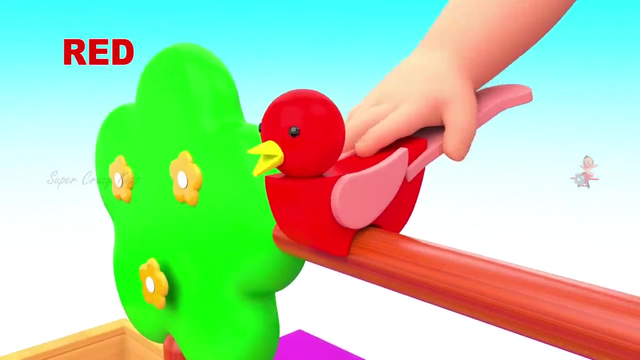 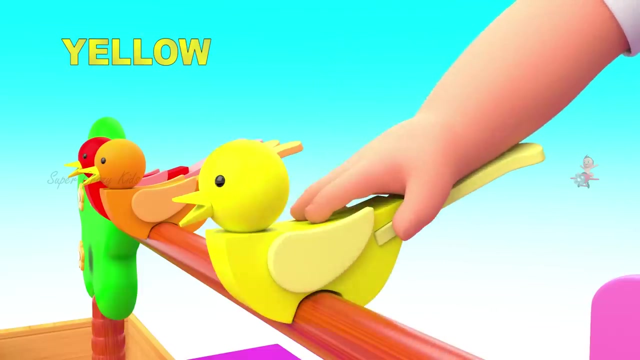 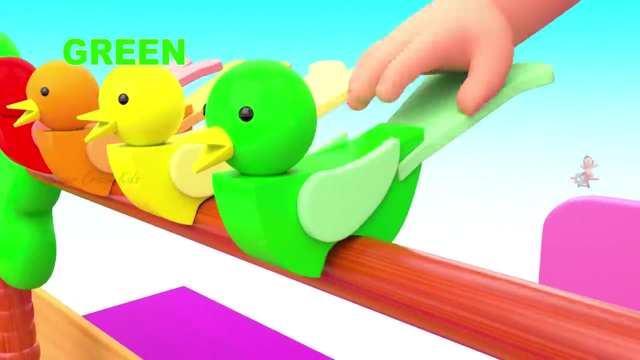 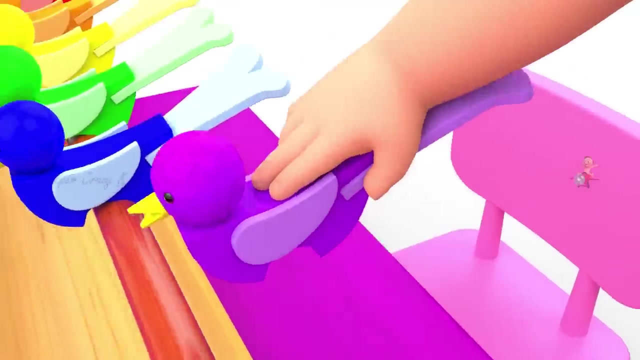 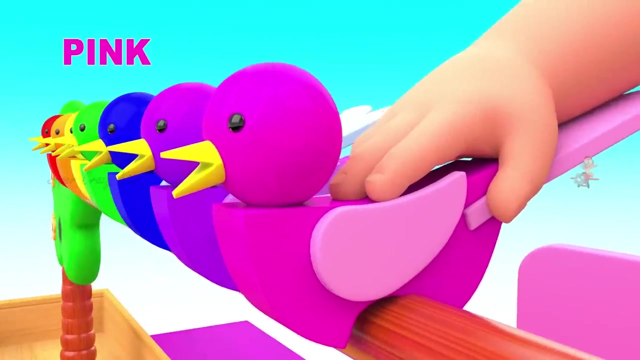 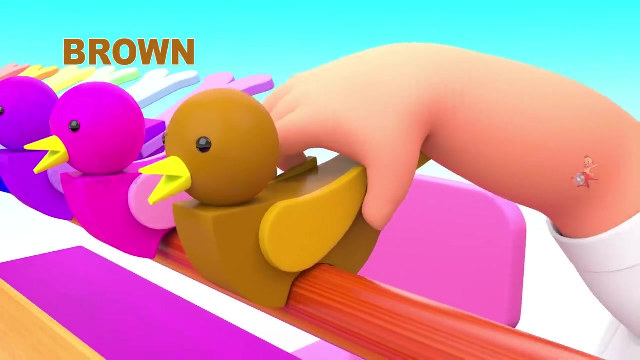 English Subtitles are available. Please click the CC button at the bottom right of the video to watch the English Subtitles. English Subtitles are available. Please click the CC button at the bottom right of the video to watch the English Subtitles. Black color. 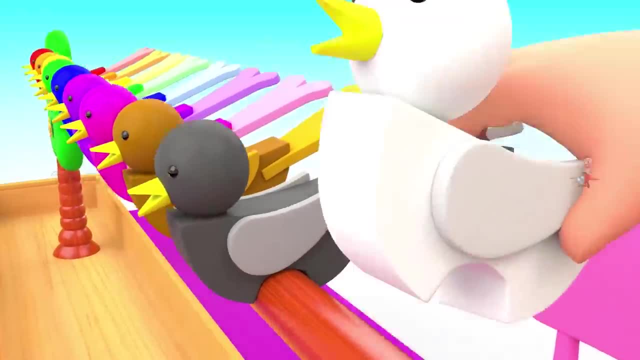 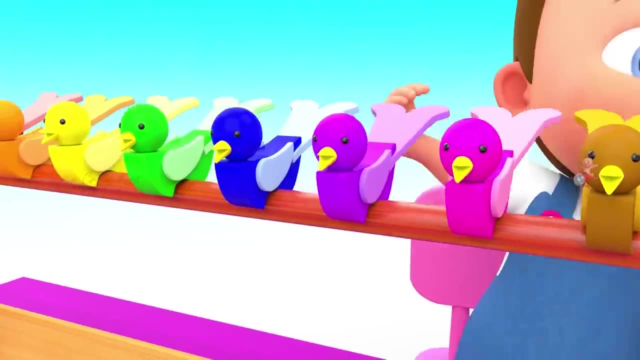 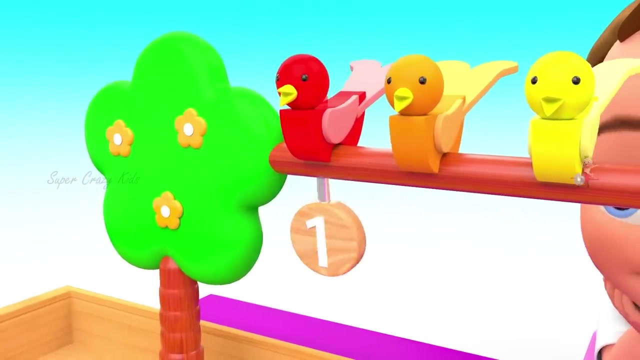 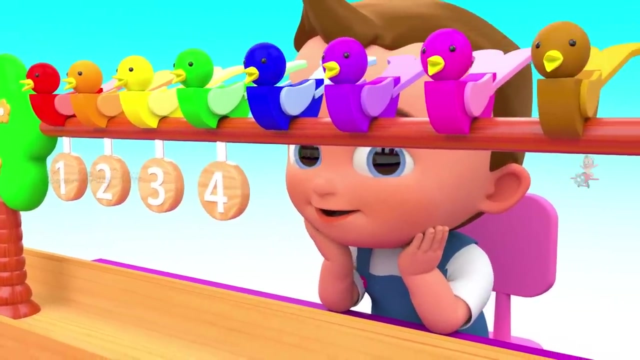 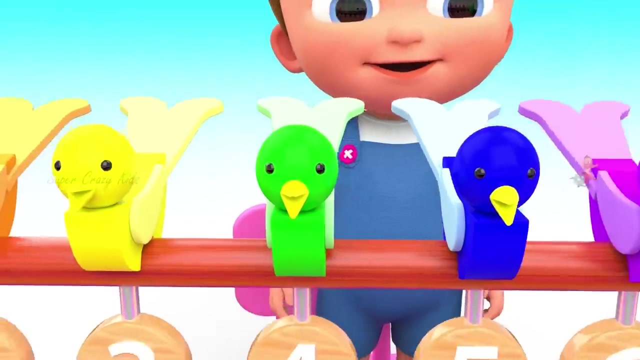 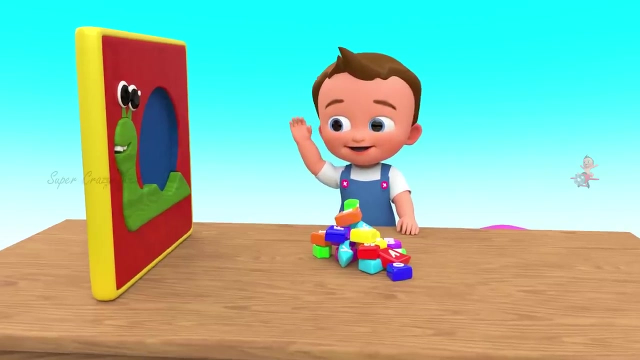 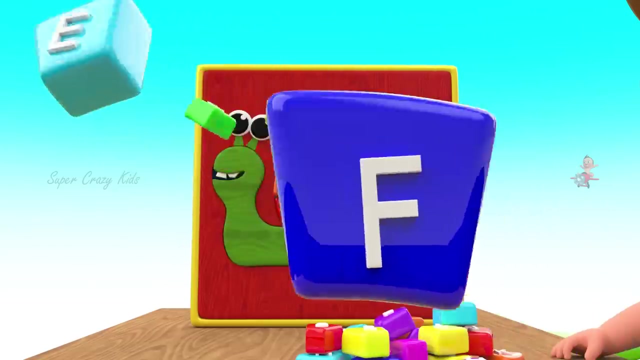 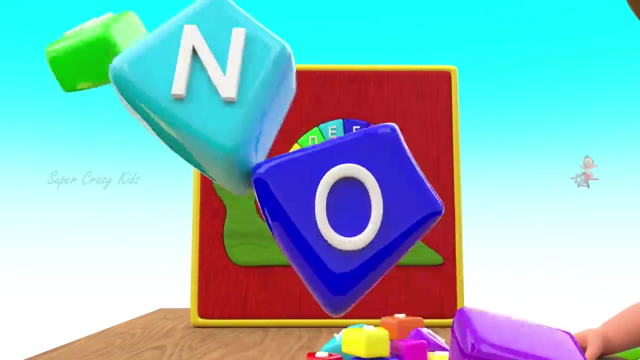 White color. One, Two, Three, Four, Five, six, seven, eight, nine, ten A, B, C, D, E, F, G, H, I, J, K, L, M, N, O P. 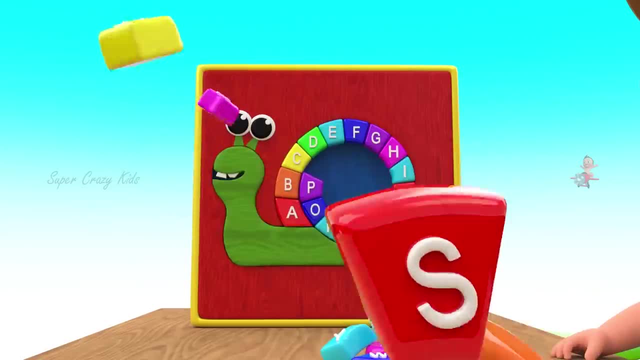 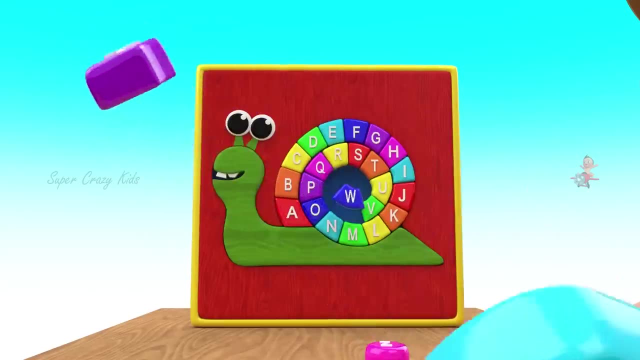 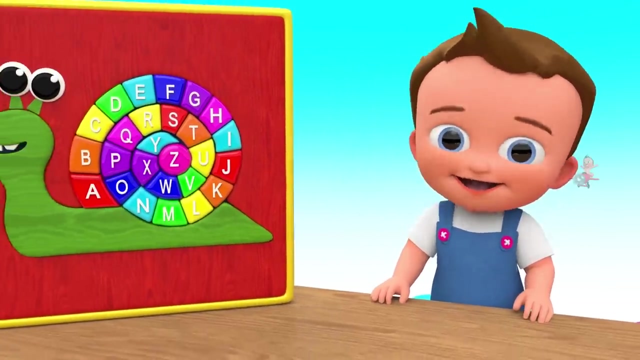 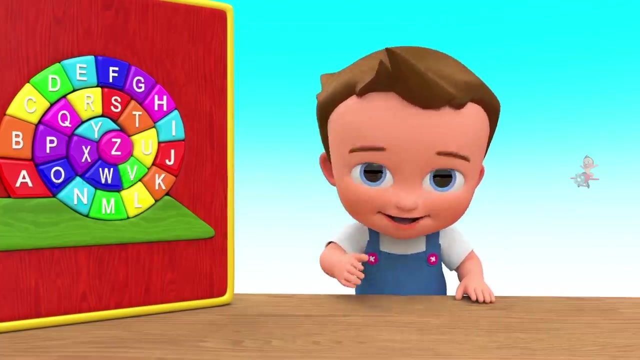 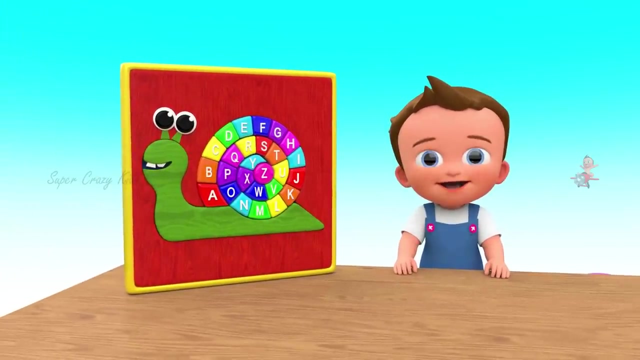 Q R, S, T, U, V, W, X, Y and Z. Now I know my A, B, Z. Next time won't you sing with me? A, A, O, R, X, Y and Z. 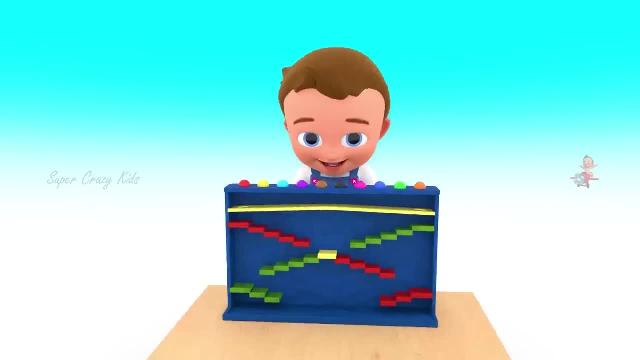 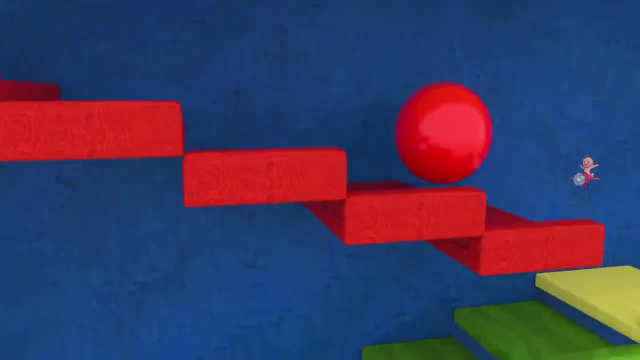 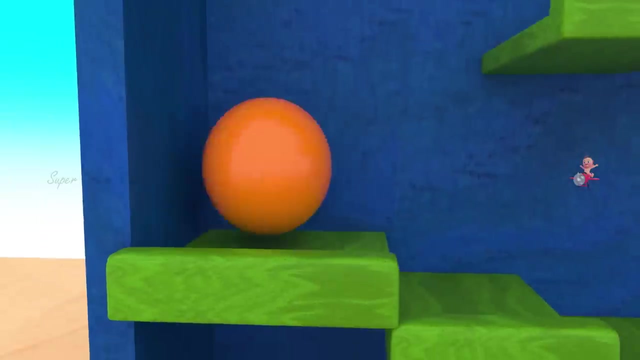 A A O R X Y and Z. A A O R X Y and Z Red color. A A O R X Y and Z Orange color. 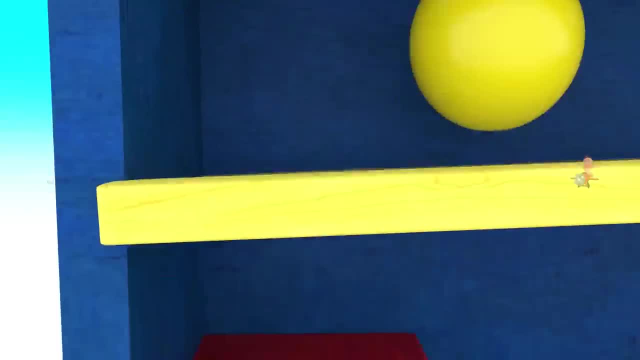 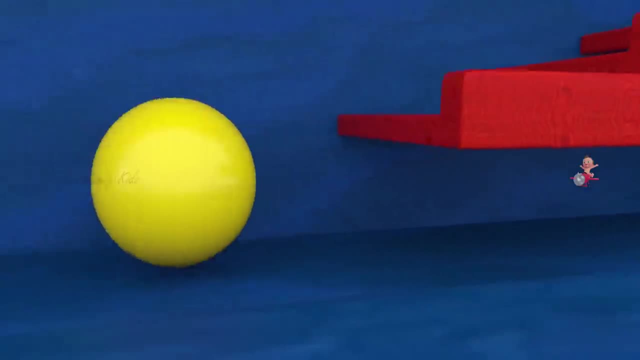 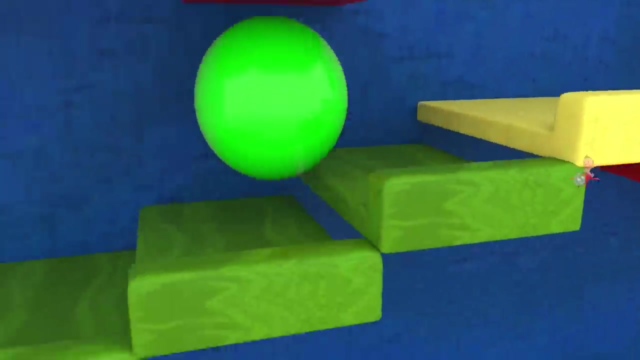 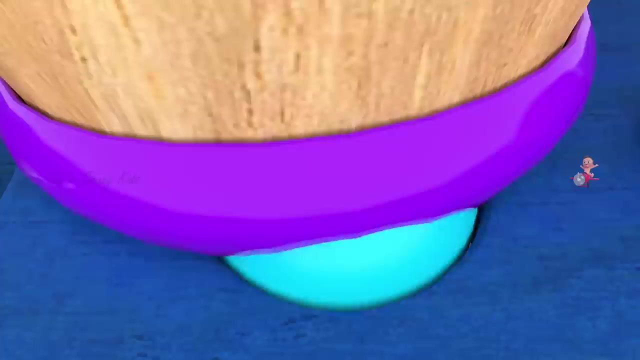 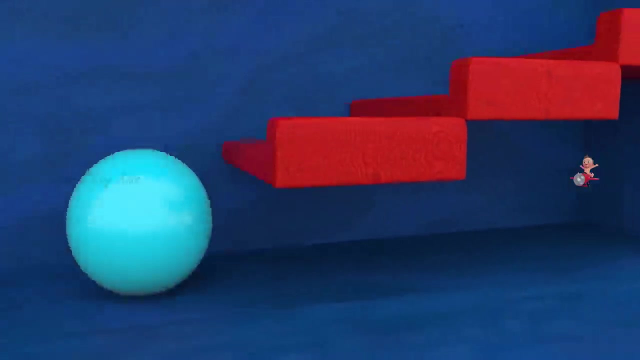 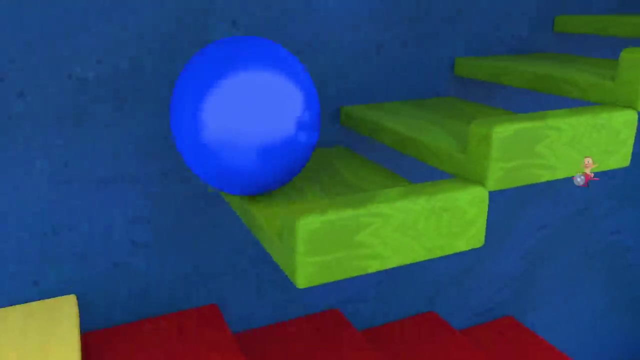 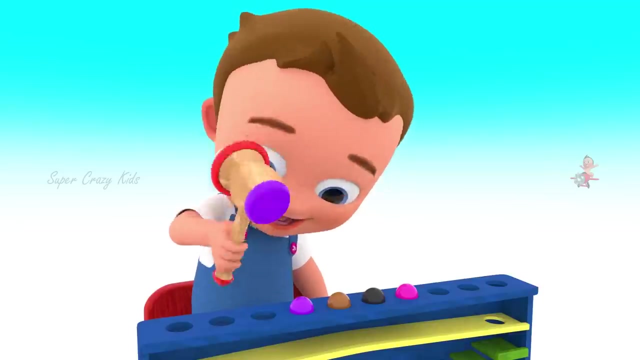 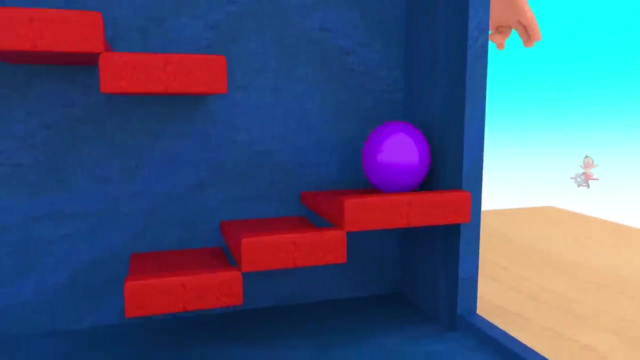 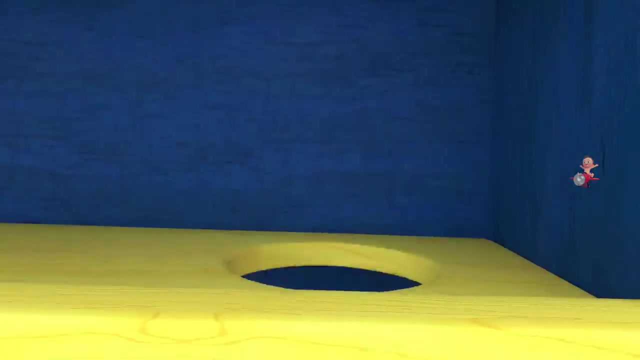 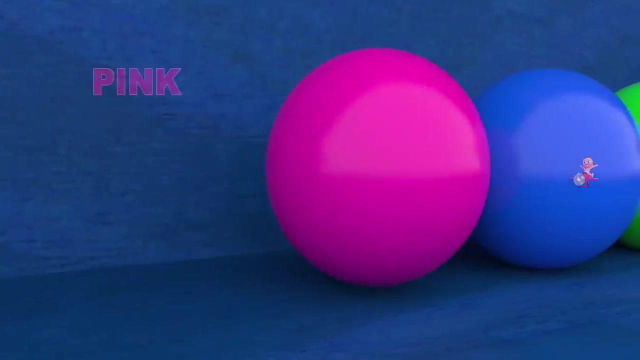 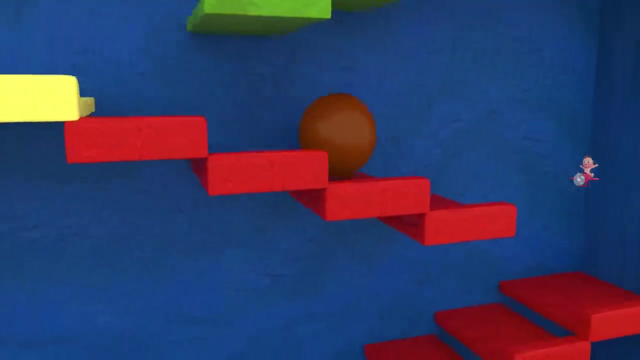 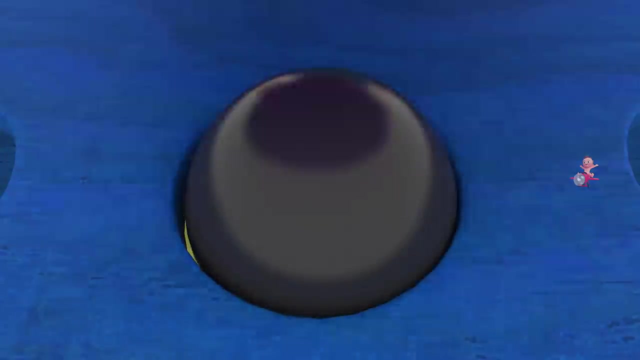 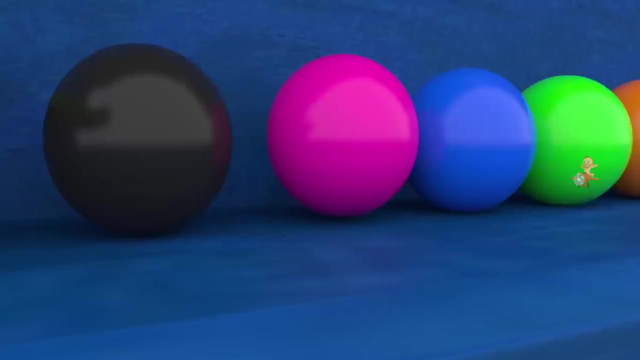 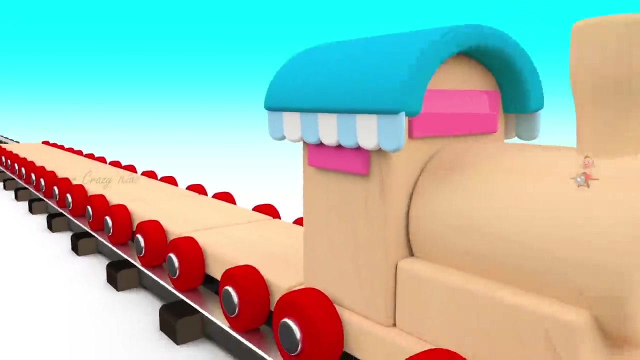 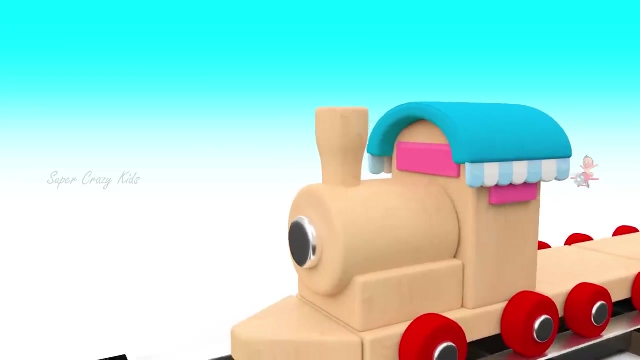 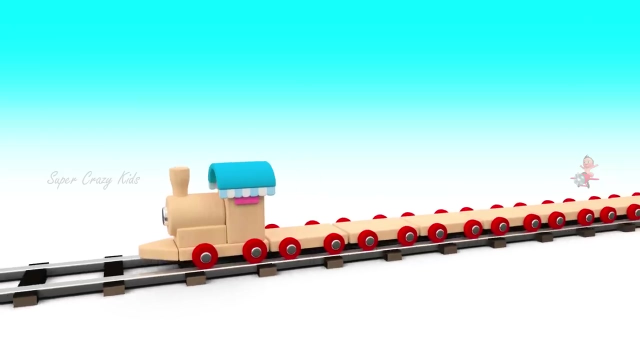 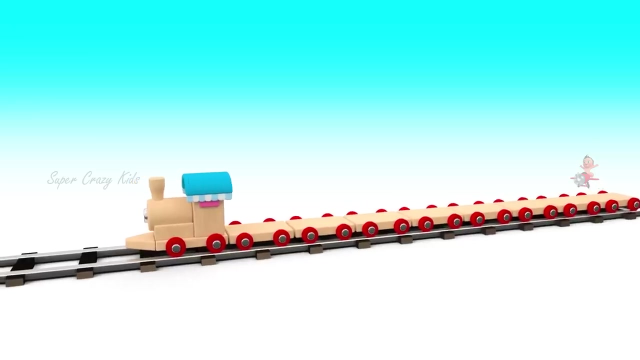 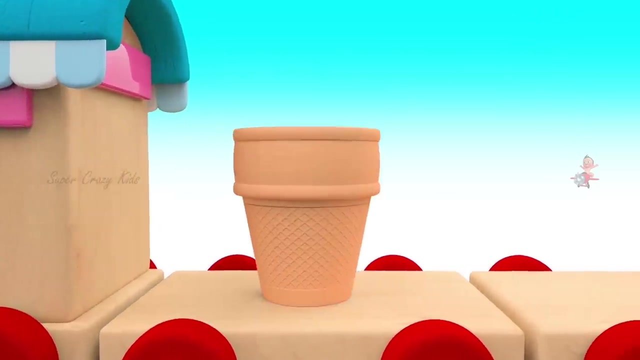 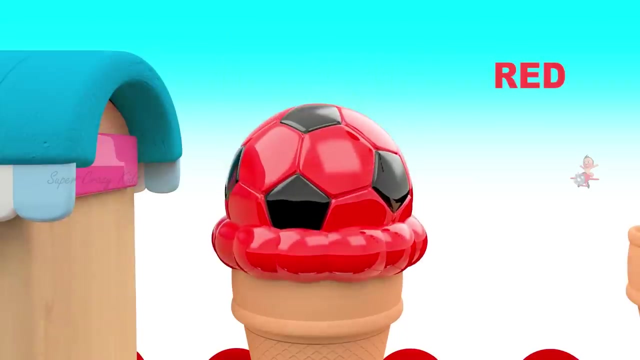 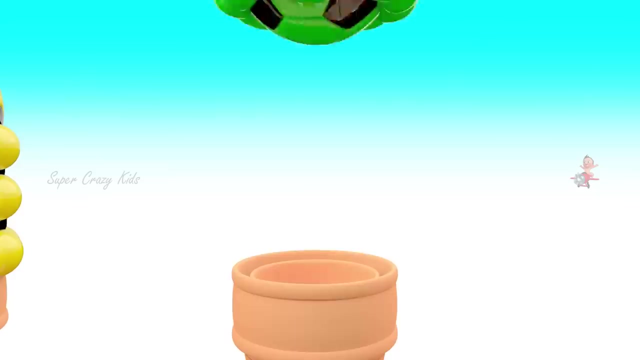 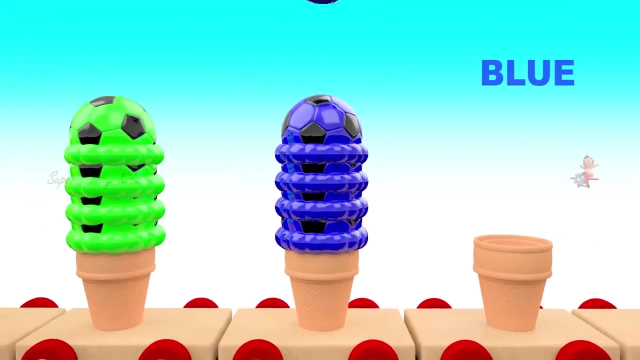 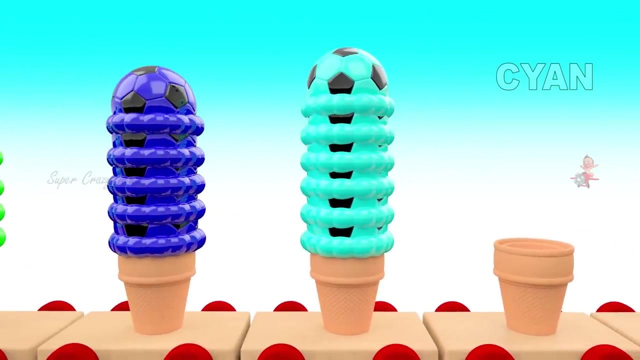 Yellow color Green color Yellow color Yellow color, Blue color Blue color, Blue color, Purple color, Pink color, Brown color, Black color Red color, Orange color, Yellow, color, Green color, Blue color, Cyan color. 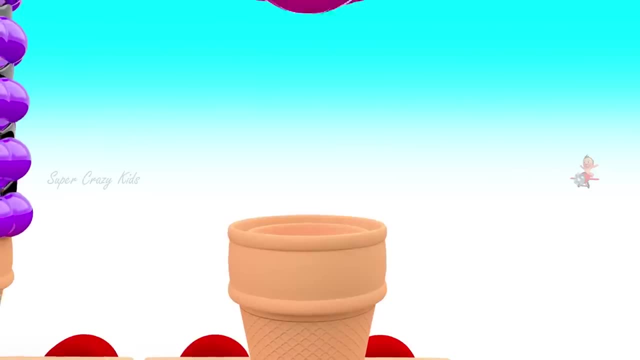 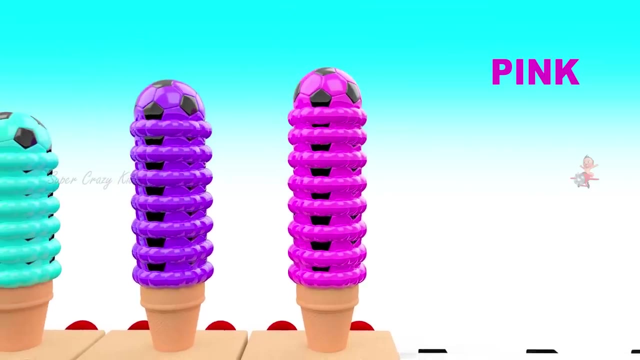 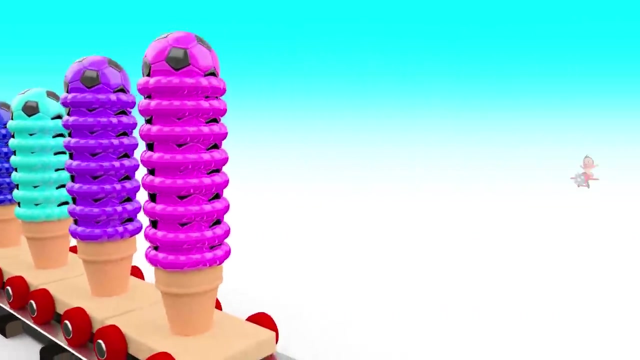 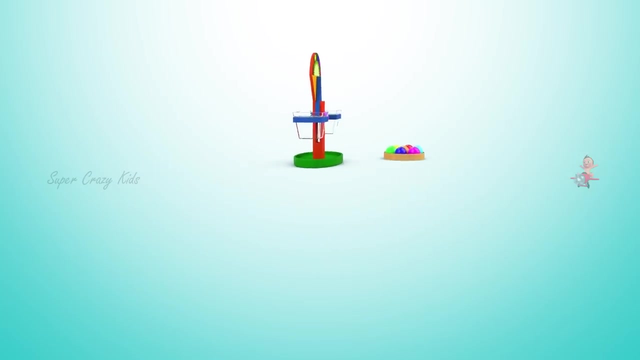 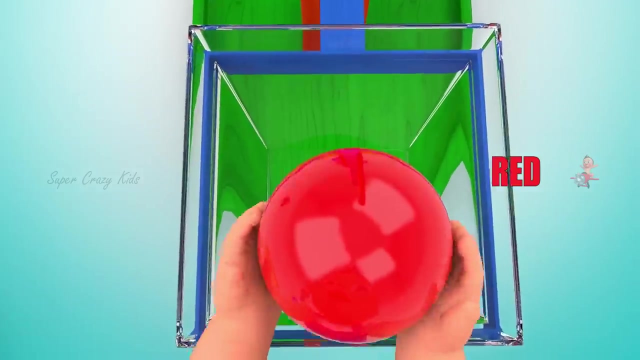 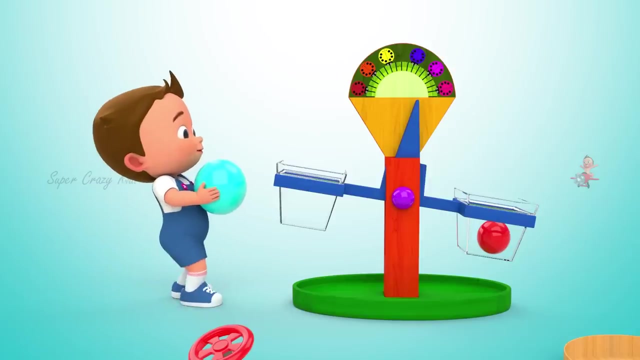 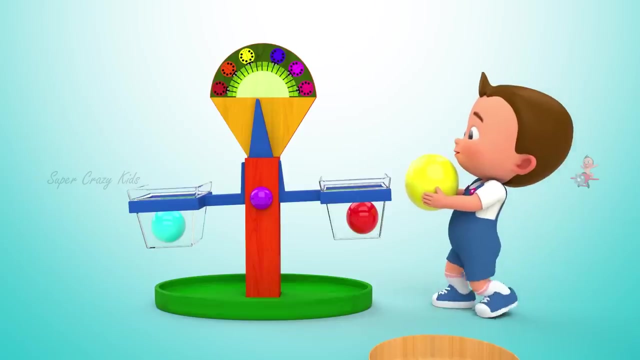 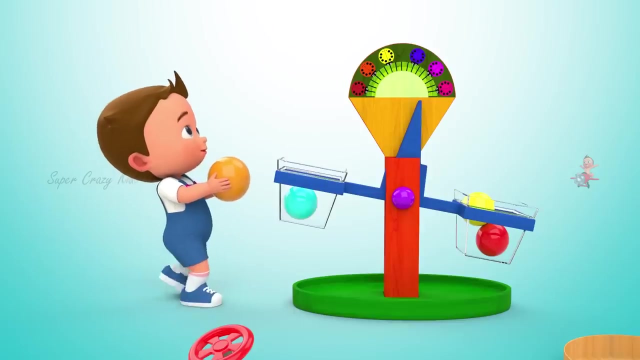 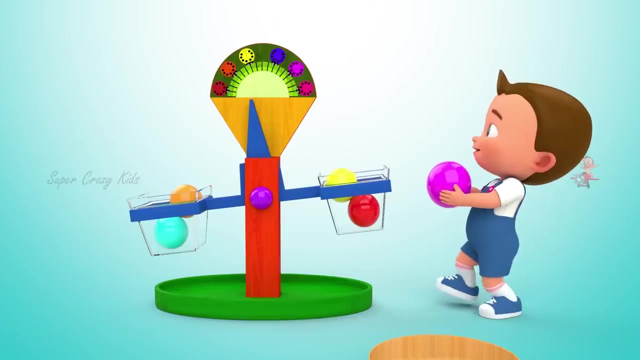 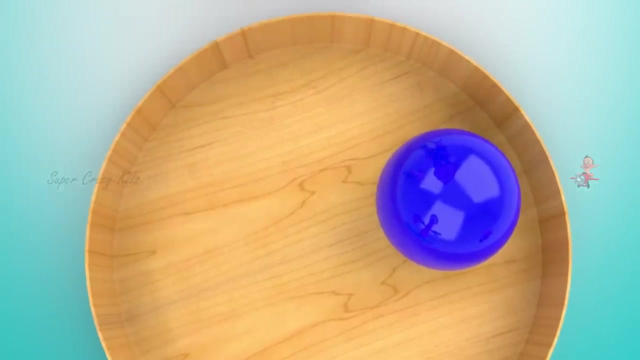 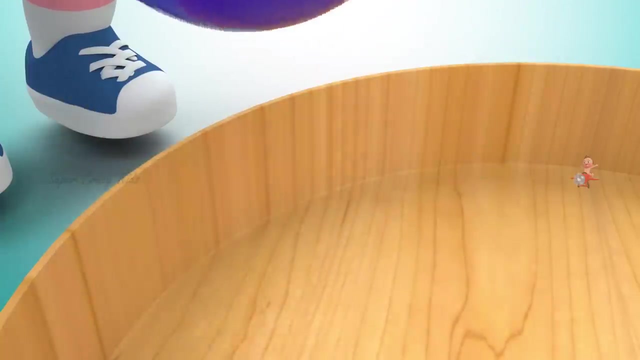 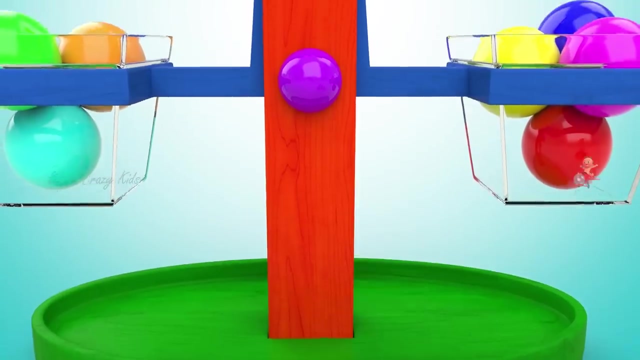 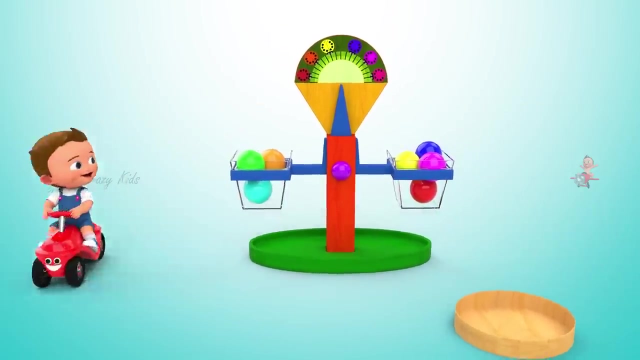 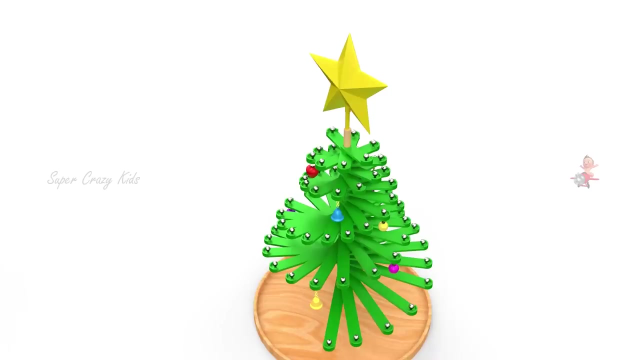 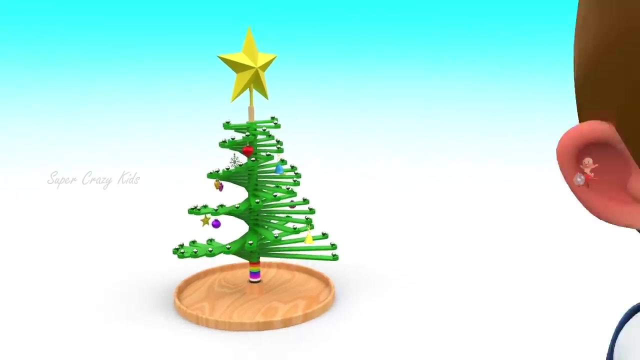 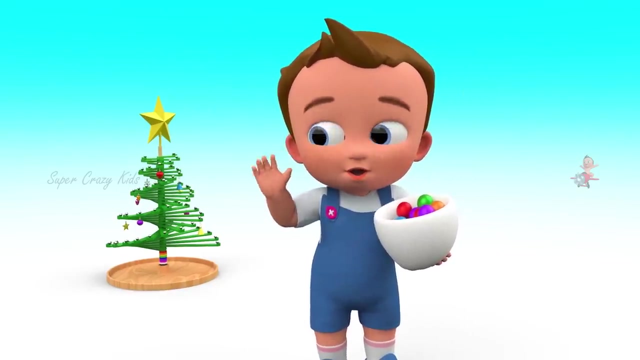 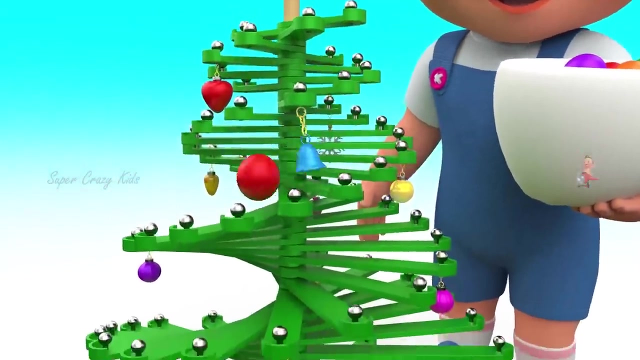 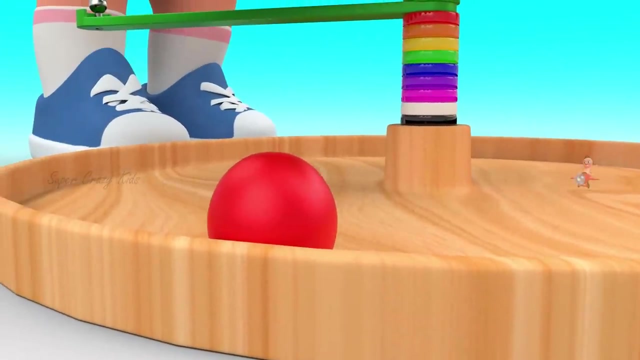 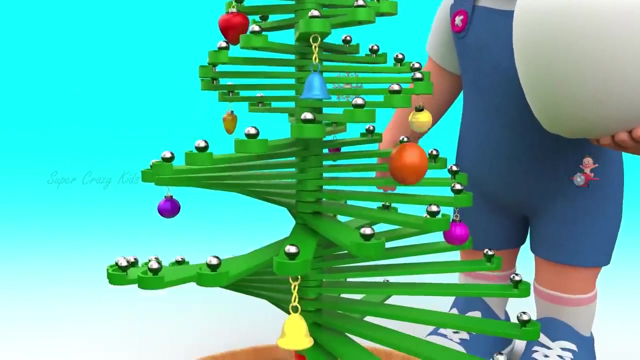 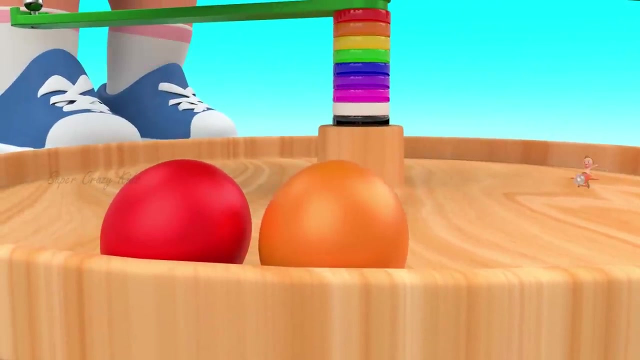 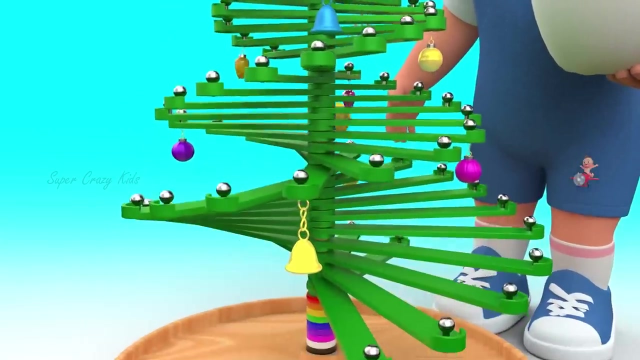 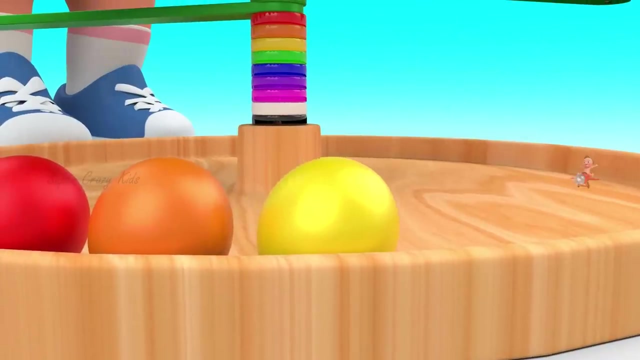 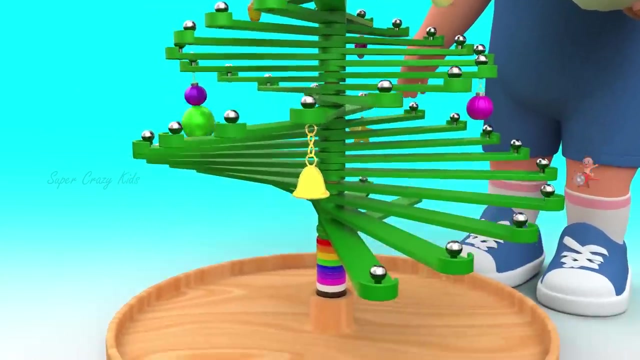 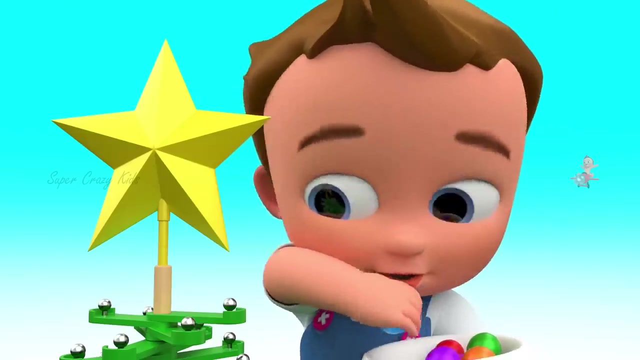 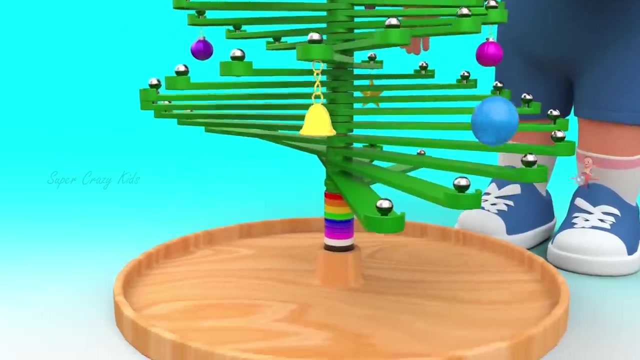 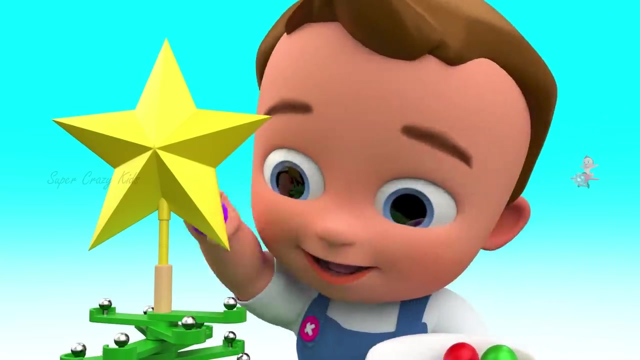 Purple color, Pink color, Red color, Red color, Cyan color, Yellow color, Orange color, Pink color, Green color, Yellow color Red color, Yellow color, Red color, White color, Blue color, White color, Blue color Orange color, Yellow color, Yellow color, Green color, Green color, Cyan color Green color. 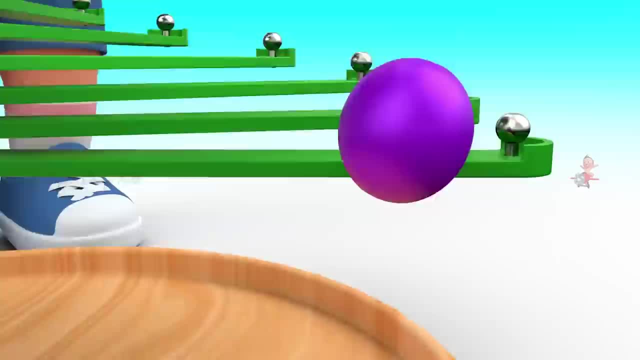 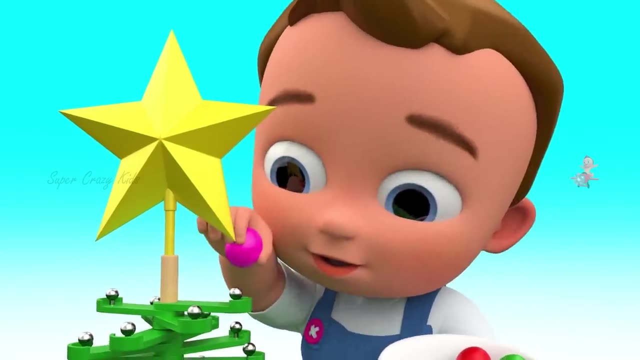 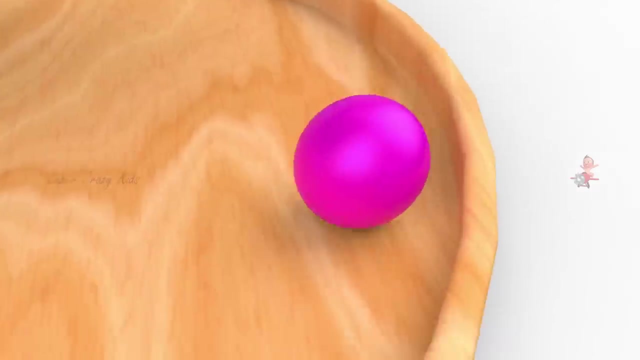 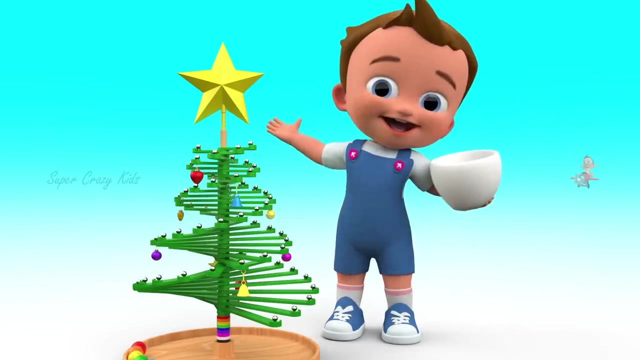 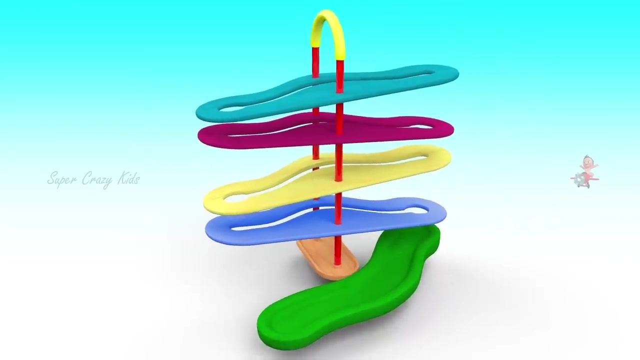 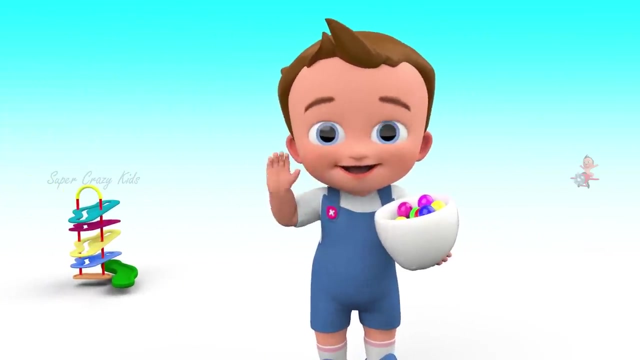 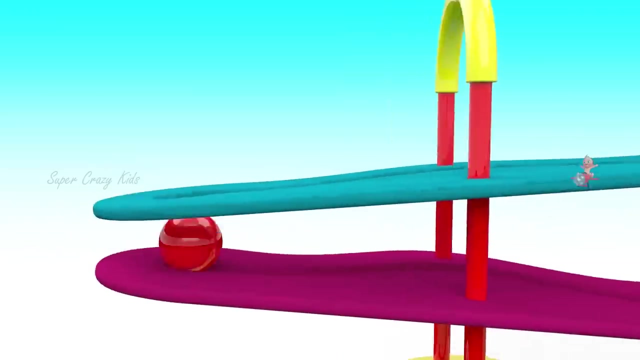 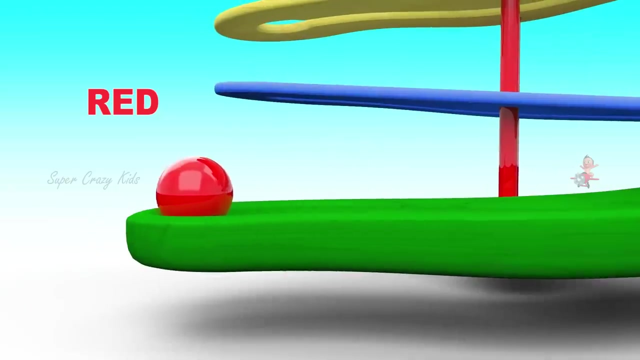 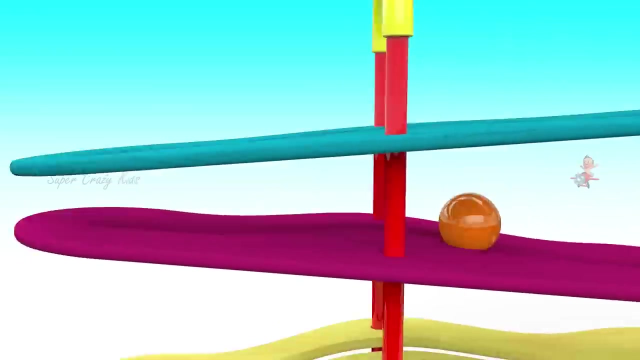 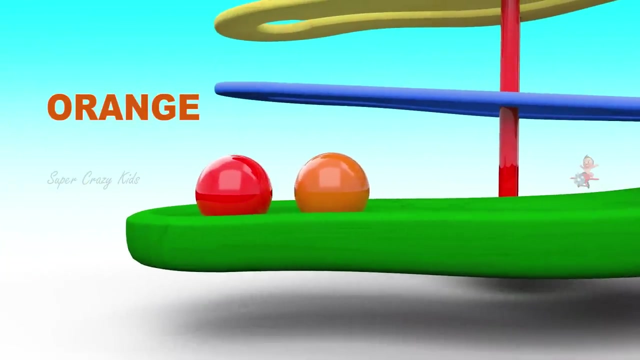 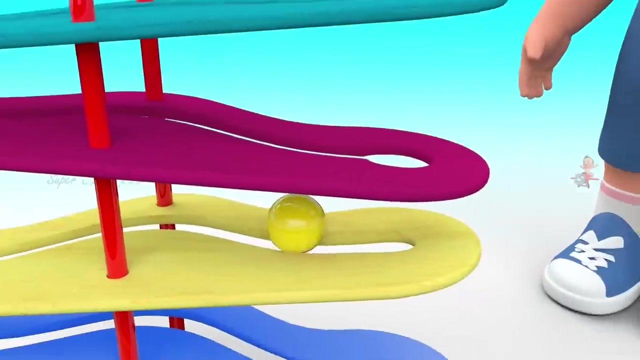 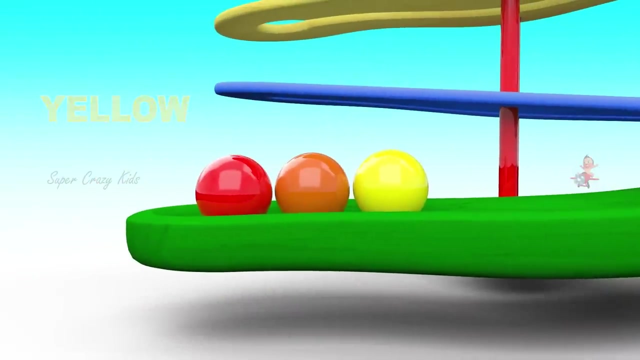 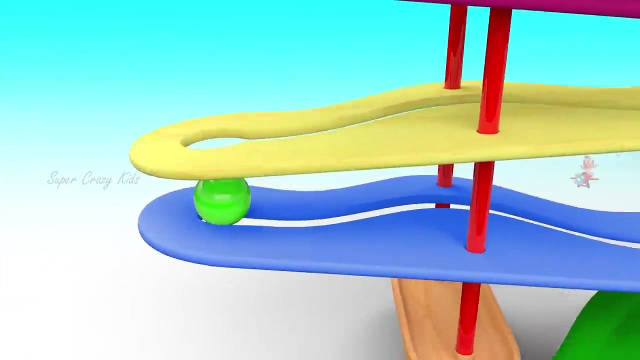 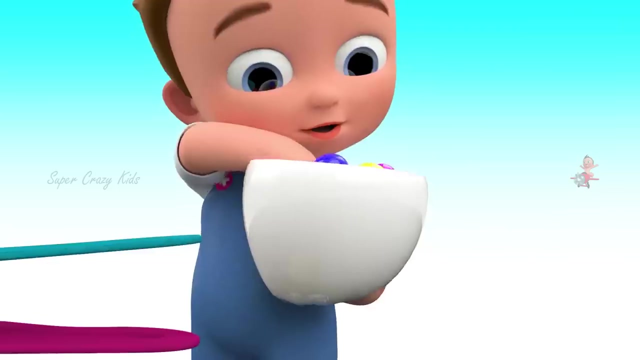 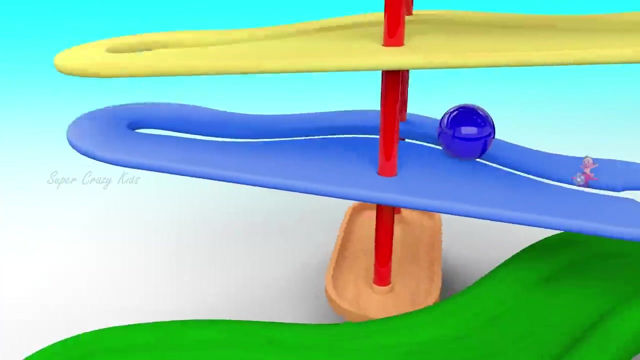 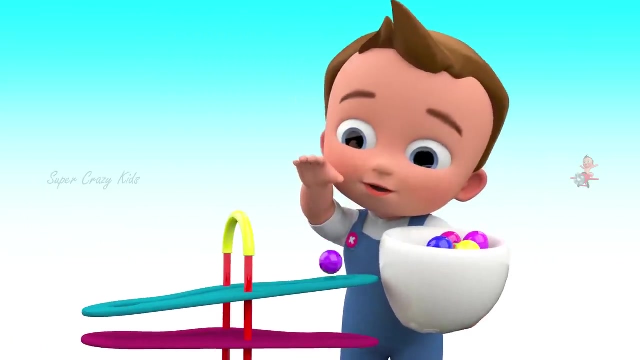 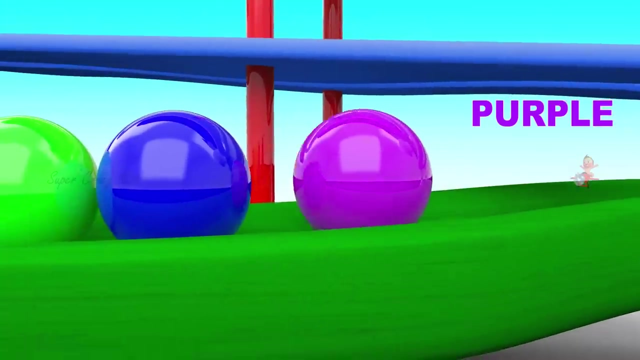 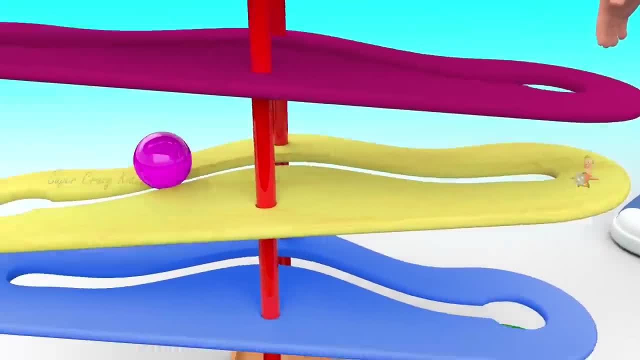 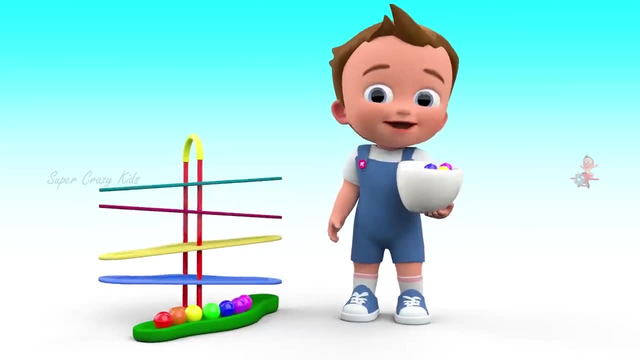 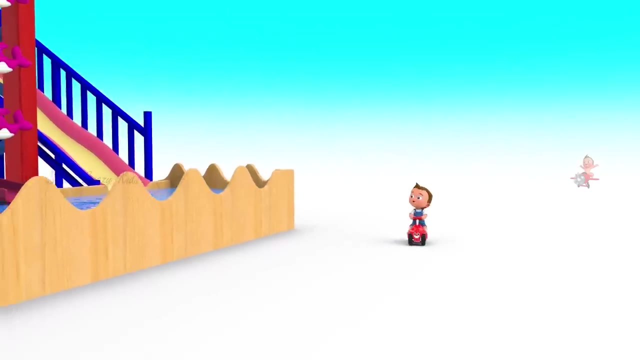 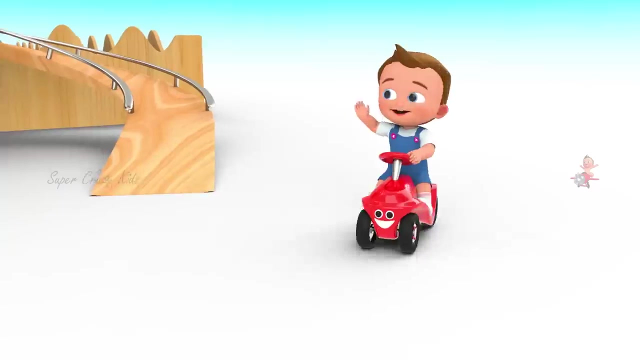 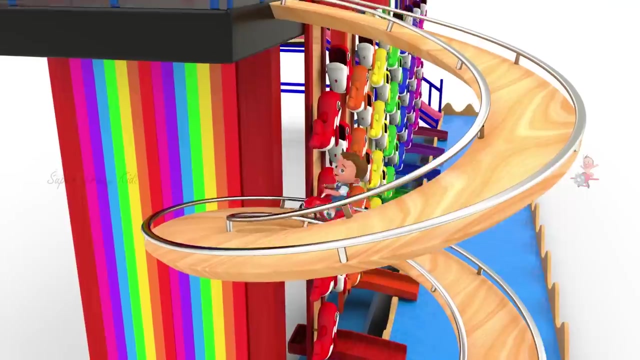 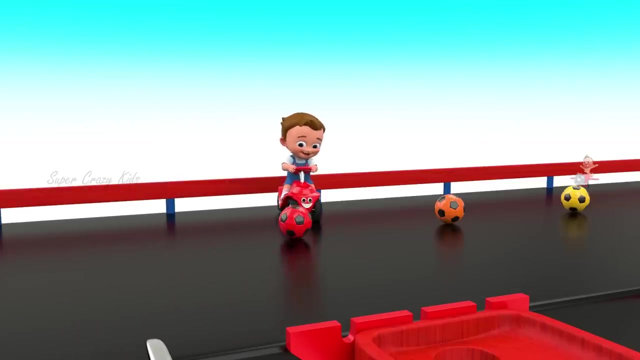 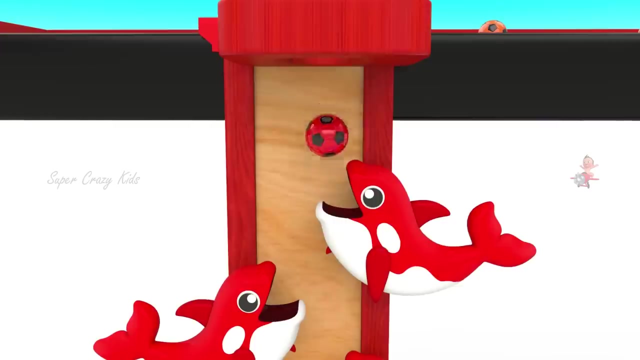 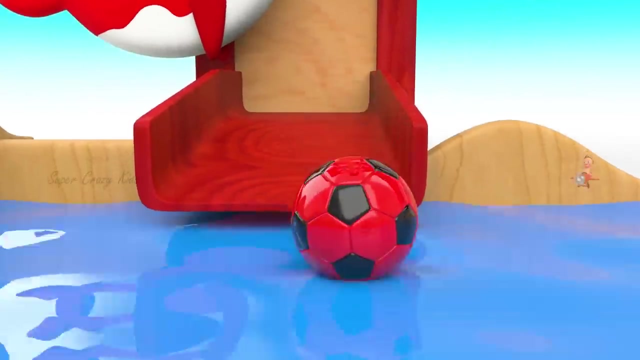 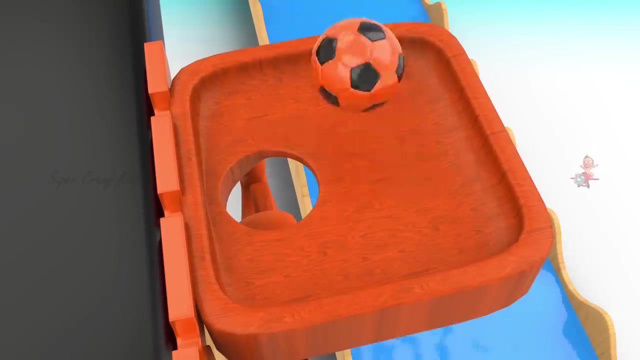 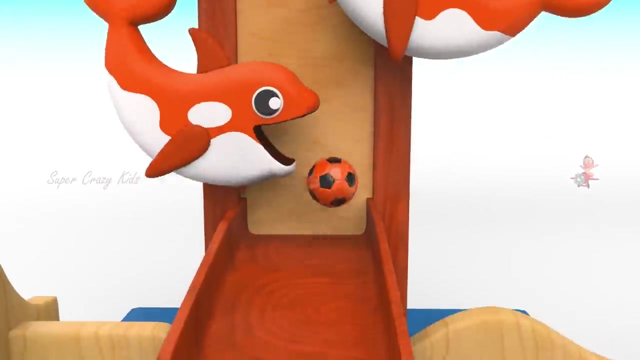 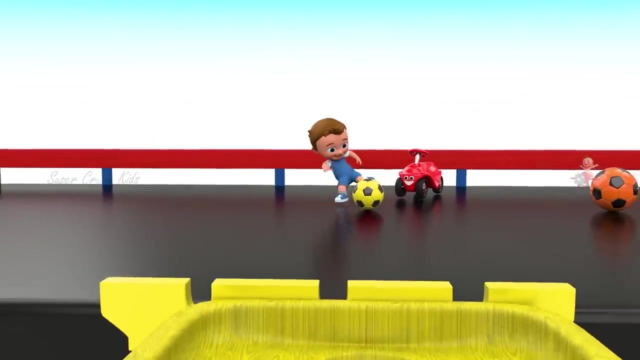 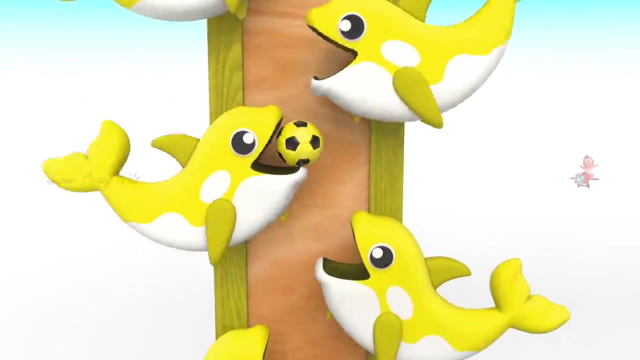 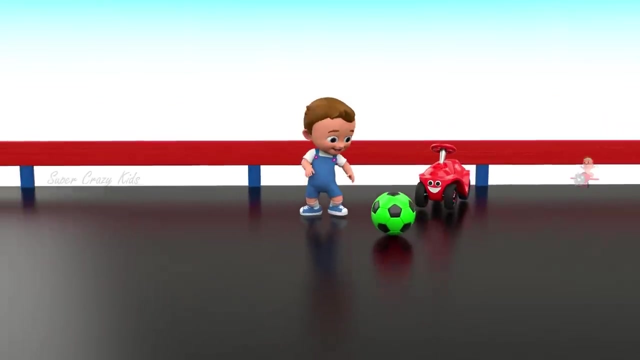 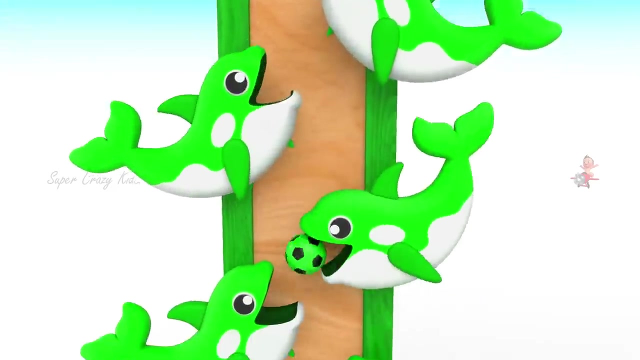 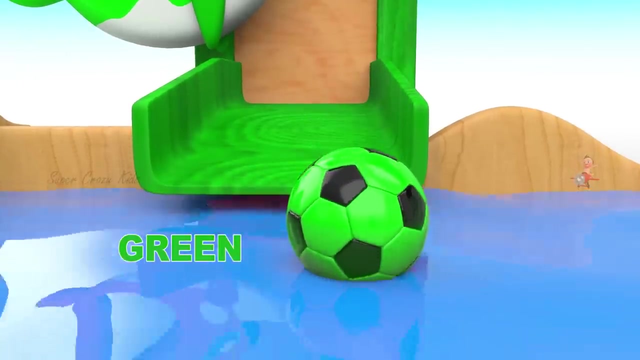 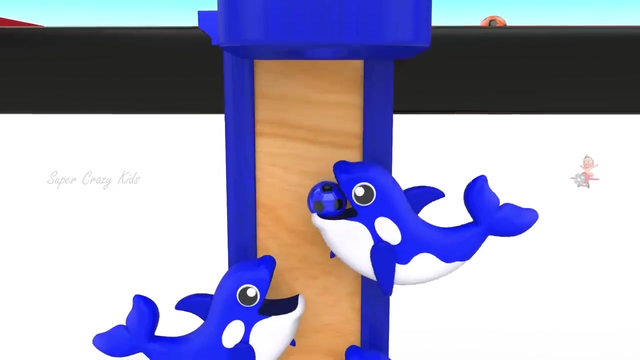 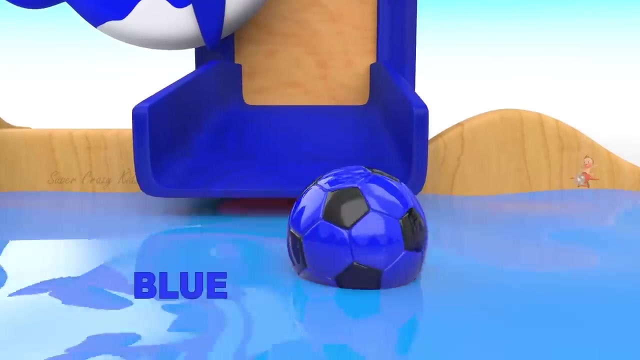 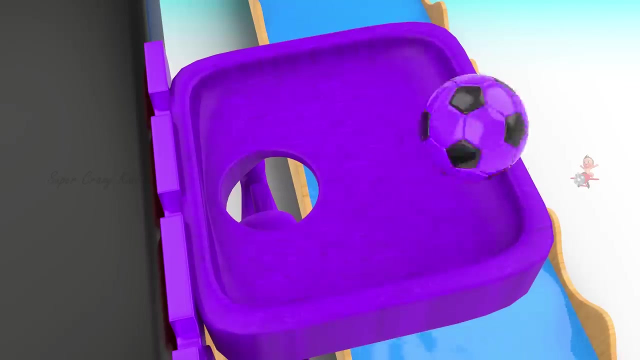 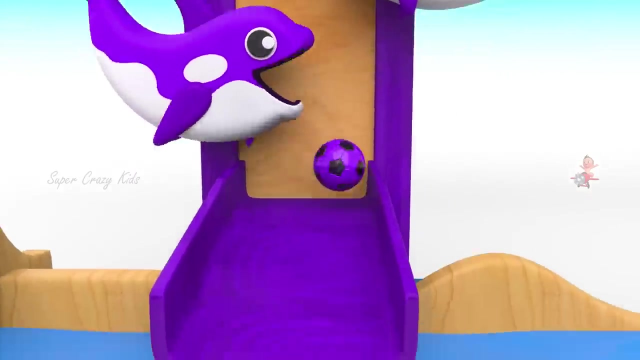 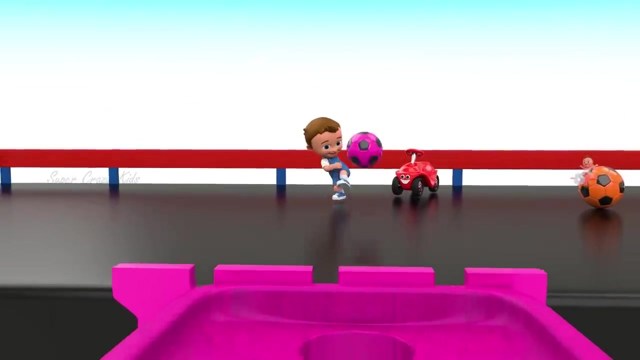 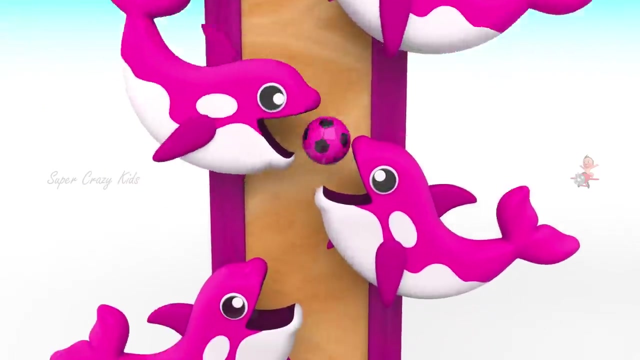 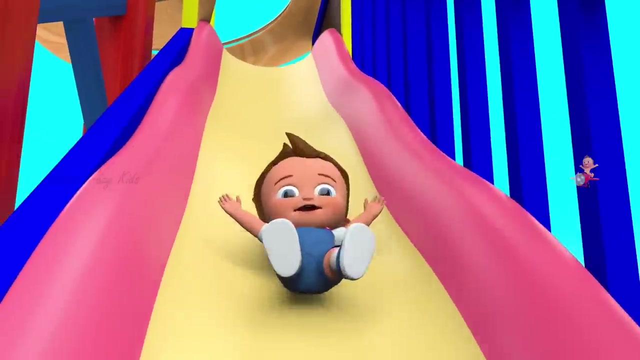 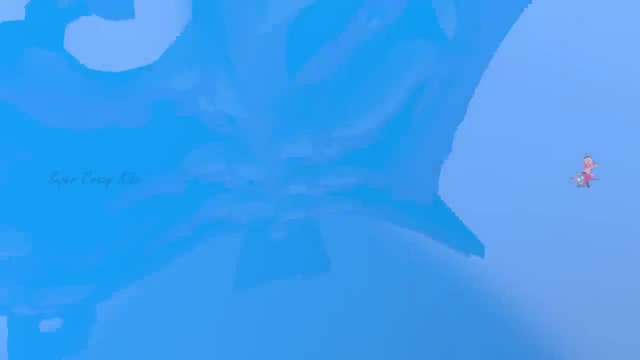 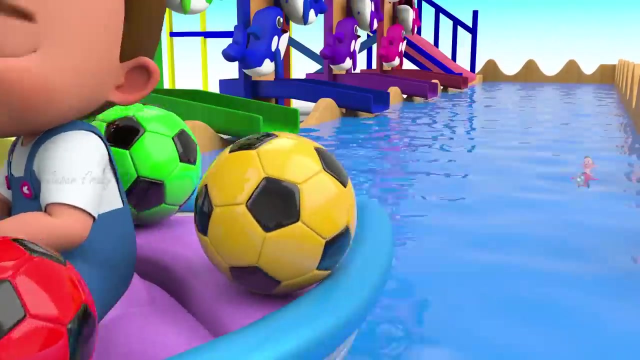 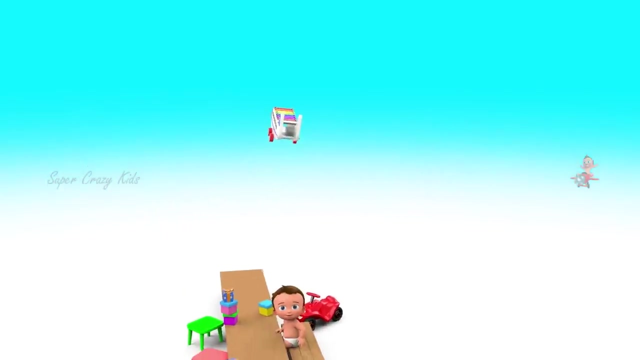 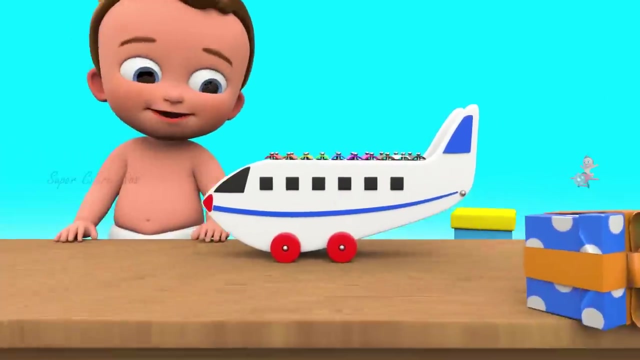 Pink color, Red color, Orange color Yellow color Green color, Blue color, Yellow color Purple color Pink color Blue color Yellow color Red color, Blue color Yellow color Red color Blue color Yellow color. 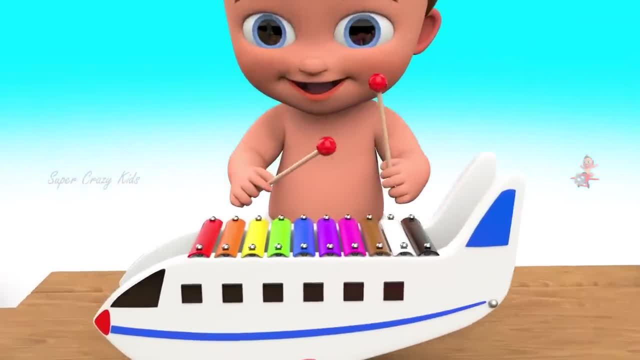 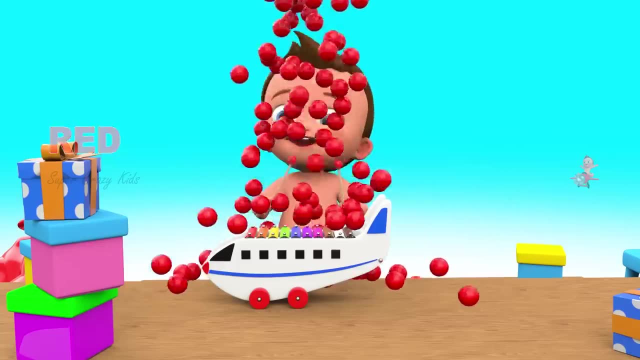 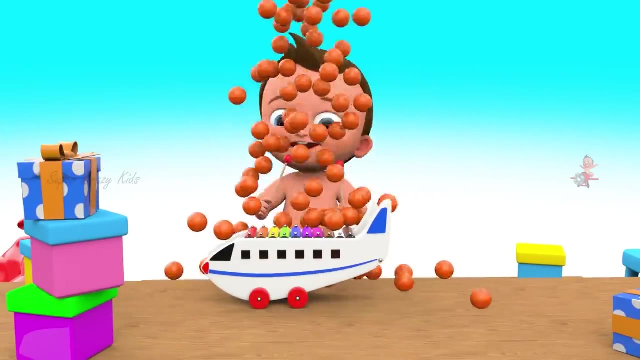 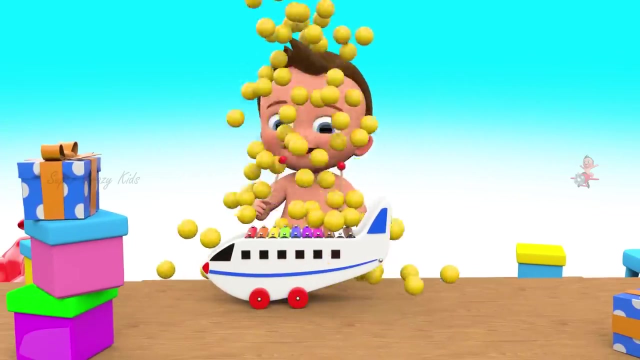 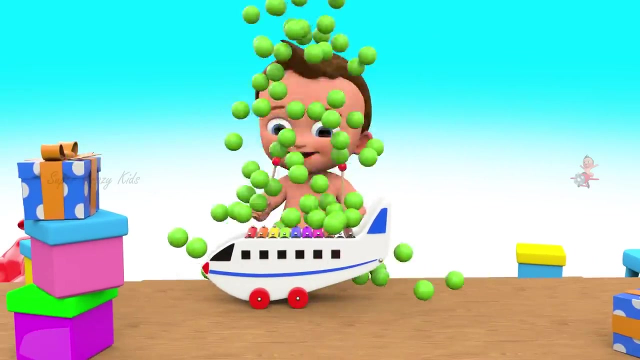 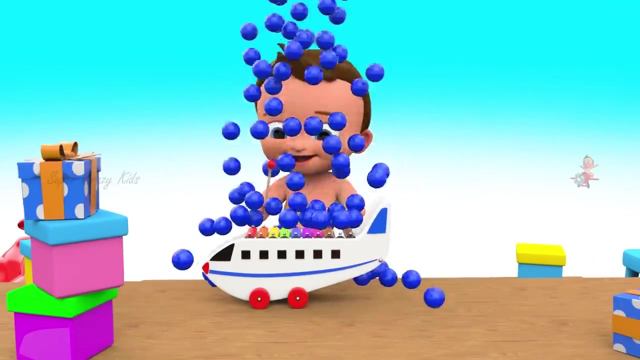 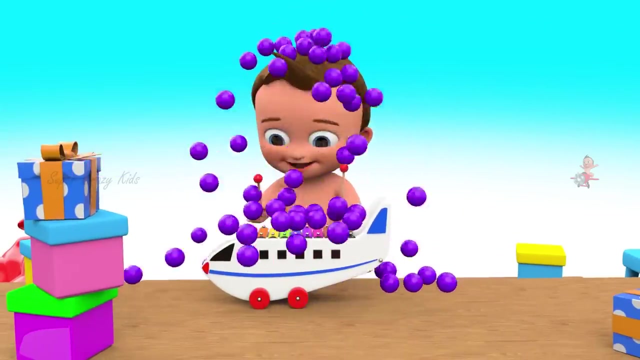 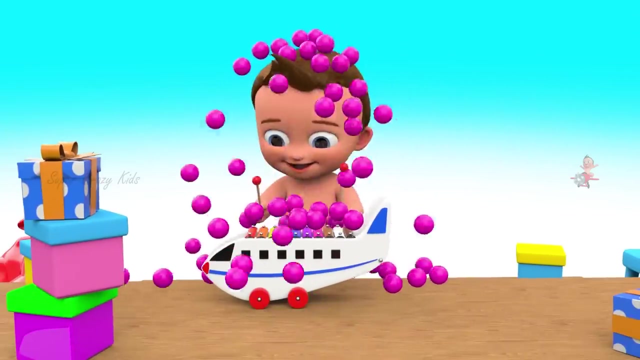 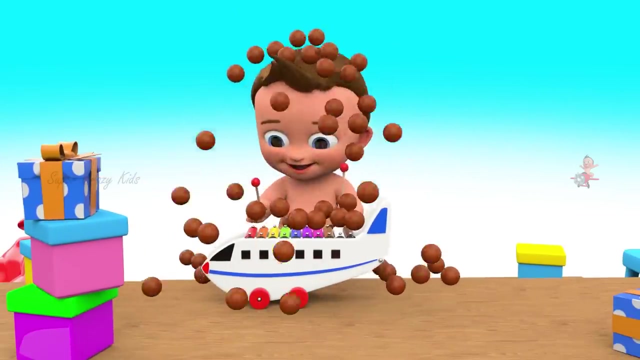 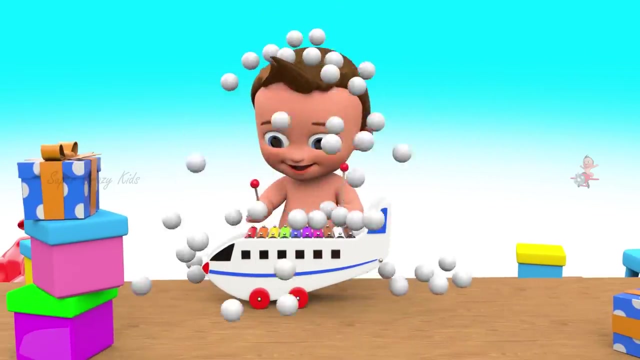 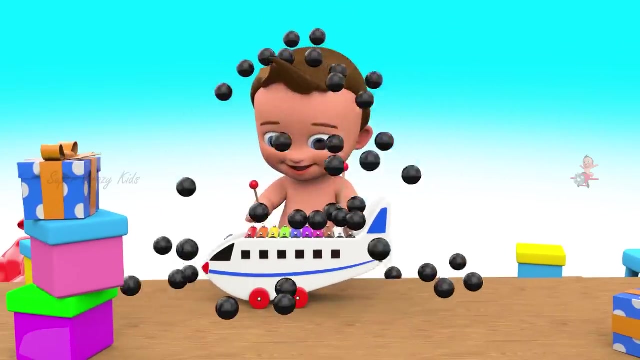 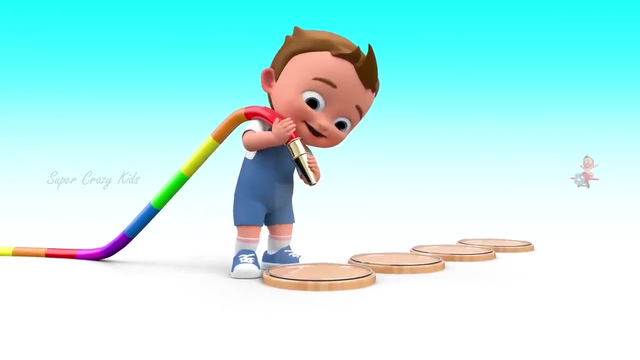 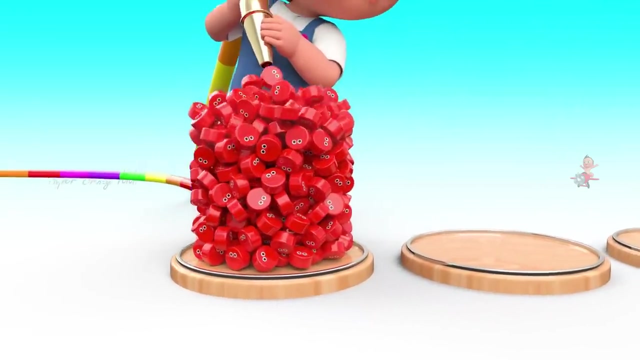 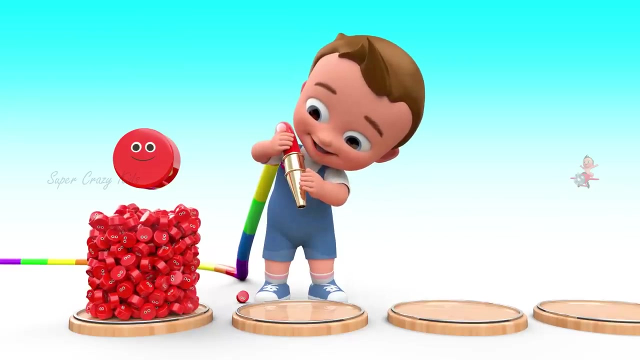 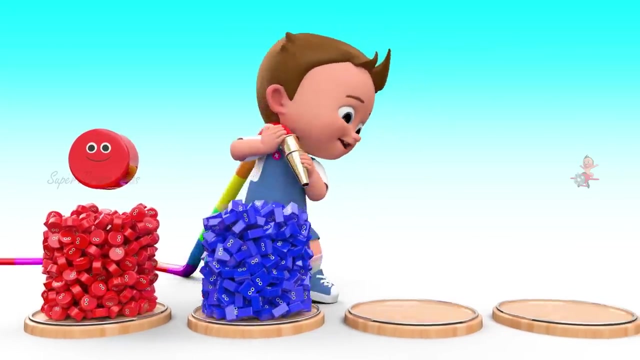 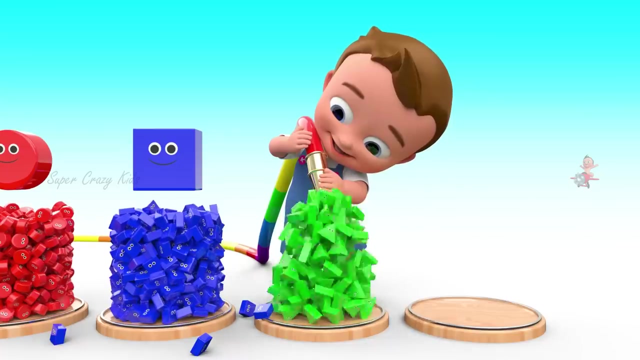 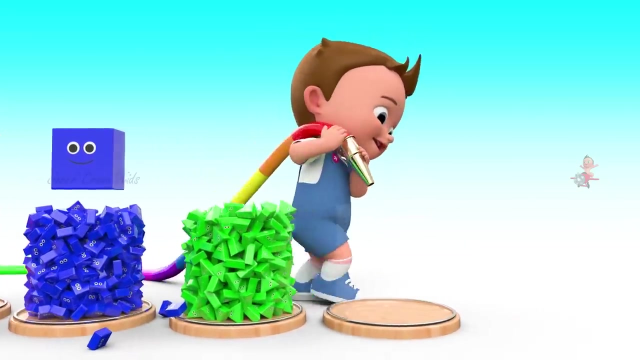 Red, color Red, color Orange, color Yellow, color Blue, color Green, color Blue, color Purple, color Pink, color Brown, color White, color Black, color Yellow, color Blue, color Circle color Square, color Triangle color. 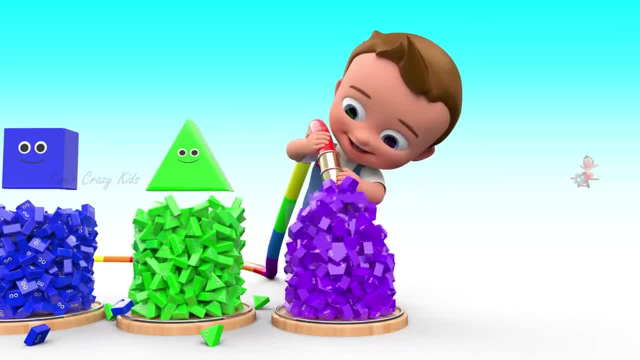 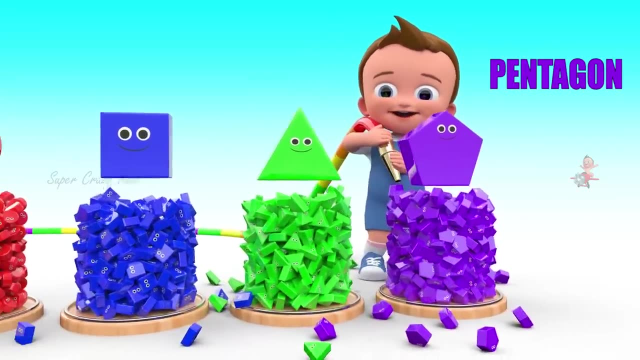 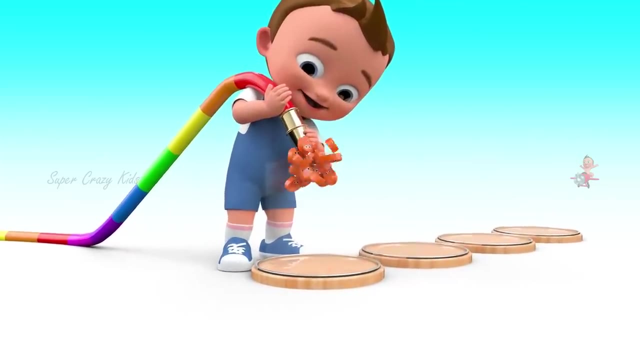 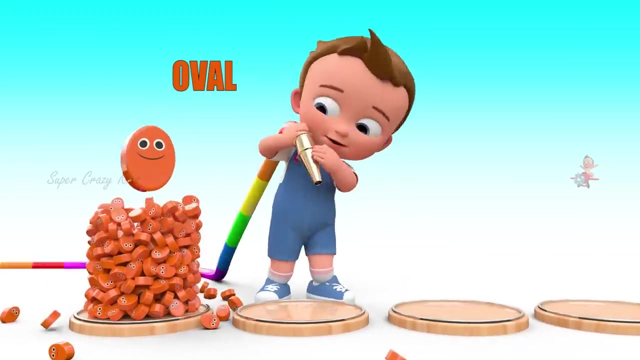 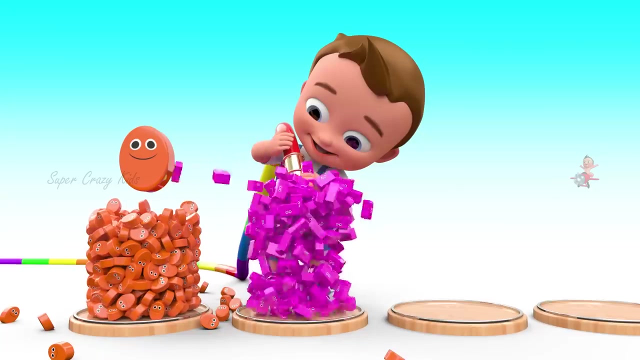 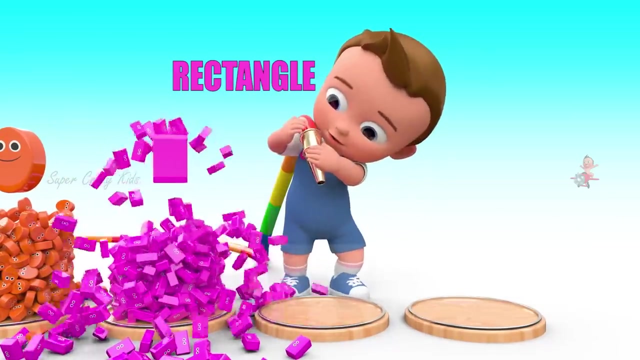 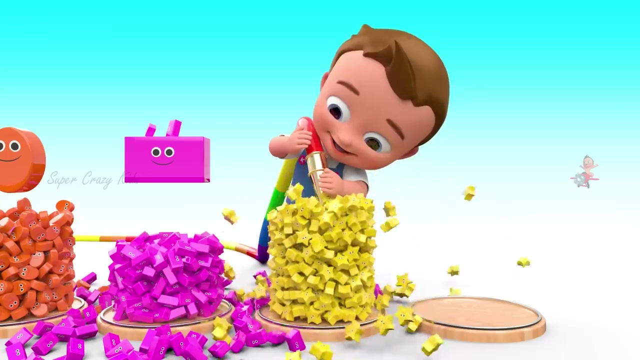 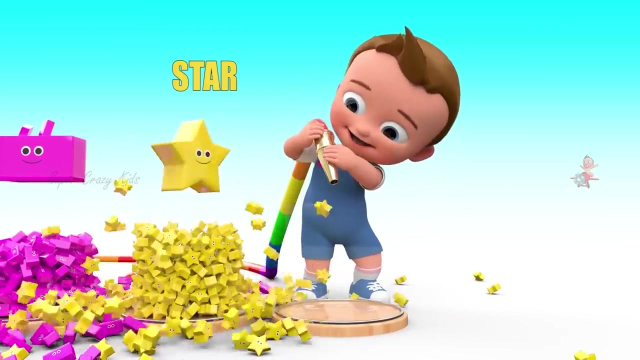 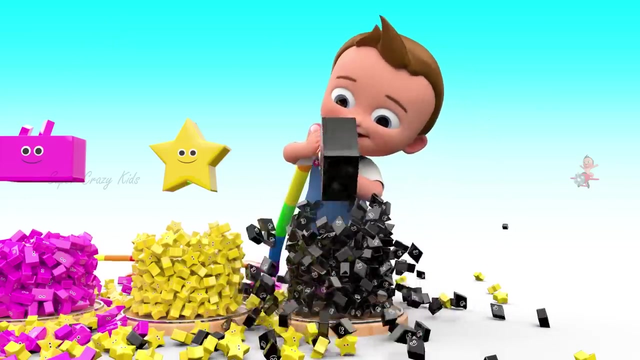 Triangle color Pentagon color Orange color Yellow color Level color. Rectangle color Star color Star color Diamond color.